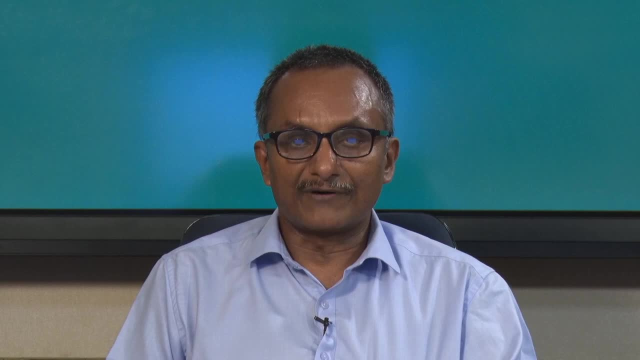 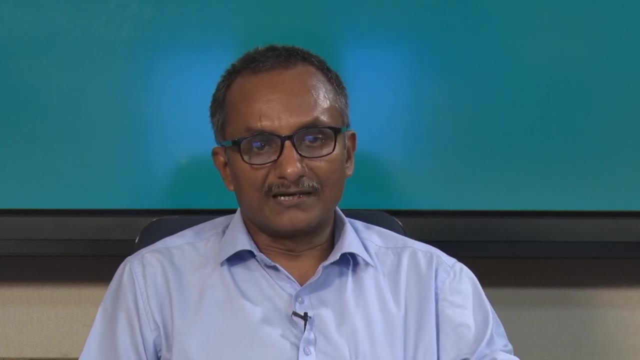 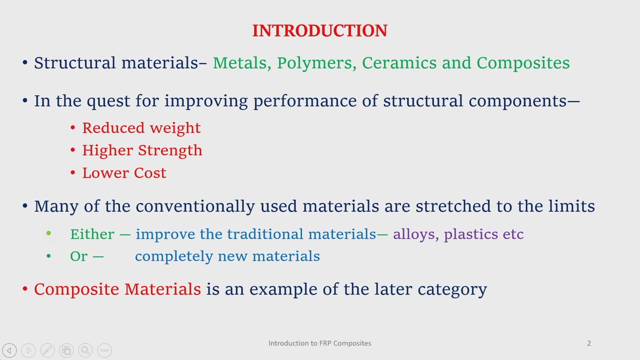 we will discuss different types of composites and FRB composites, as well as different terminologies. So to start with, we know that the structural materials basically are classified as metals, polymers, ceramics and composites. Now, with the advancement of science and technology, you know that there are the requirement 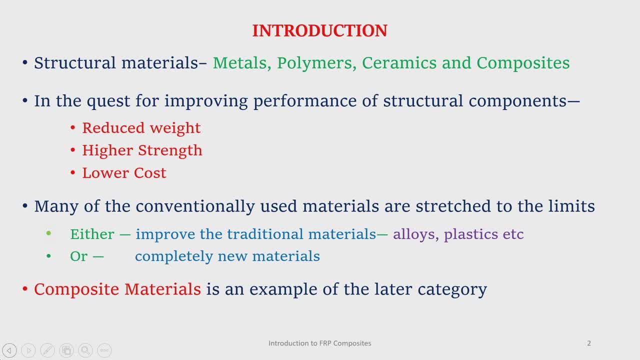 of improved performance also increased, and so the in the quest for improving the performance of structural composites say, for example, many in many aerospace applications we like to use materials so that the weight is minimized. Then in many load bearing applications we like to increase the strength. that means we want higher strength materials. Of course. 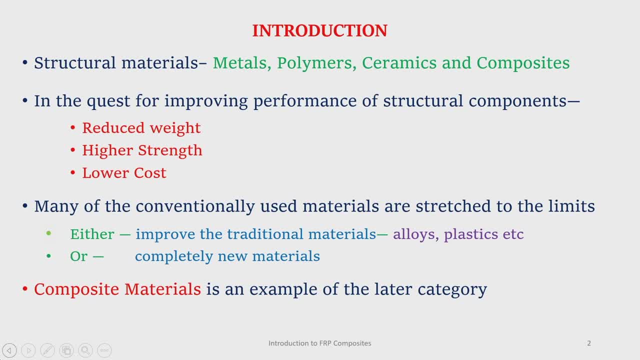 for each. for all these cases, we always like to minimize the cost. Now, in doing so, what happens is many of these conventionally used materials are actually stressed to the limits. that means there is hardly any scope of improvement. ok, So how to do this? So there are two ways: either improve the traditional materials and 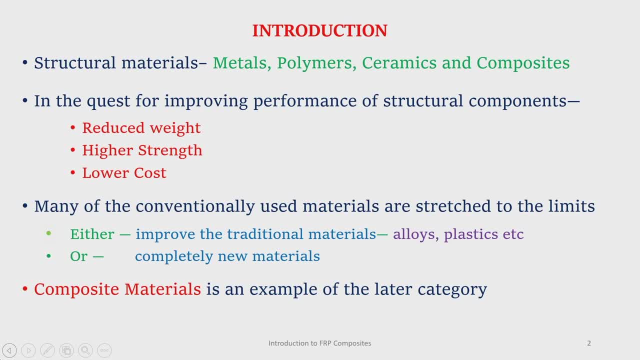 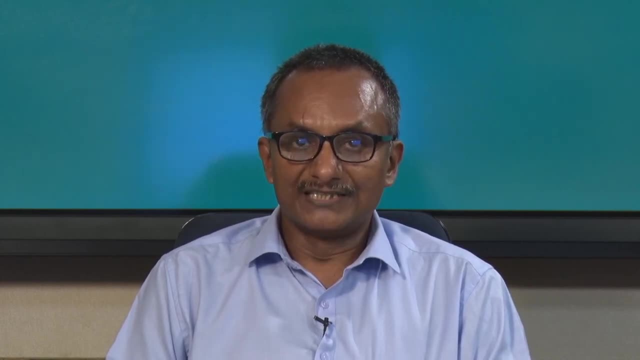 in doing so. we know that there are different types of alloys. plastics have come up, like we use alloying elements in steels to improve some of the properties, ok. or if that does not work, may be a completely new material have to be thought of. This is here the composite. 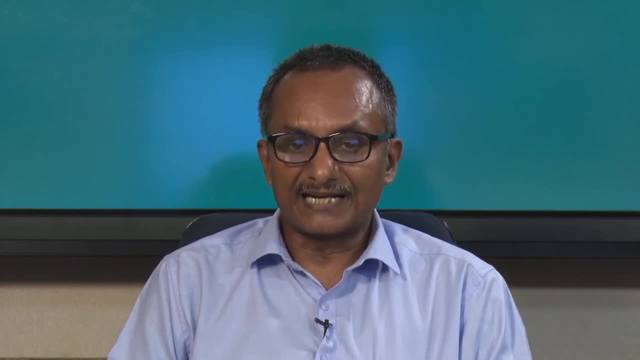 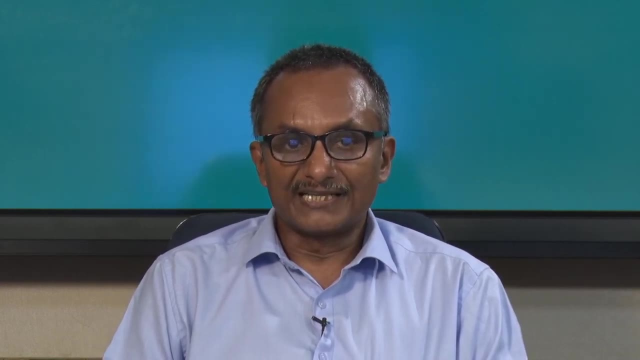 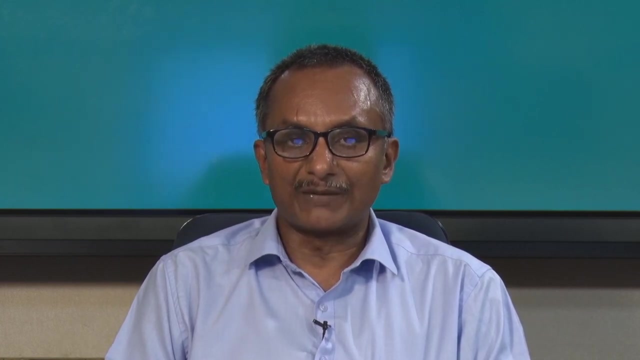 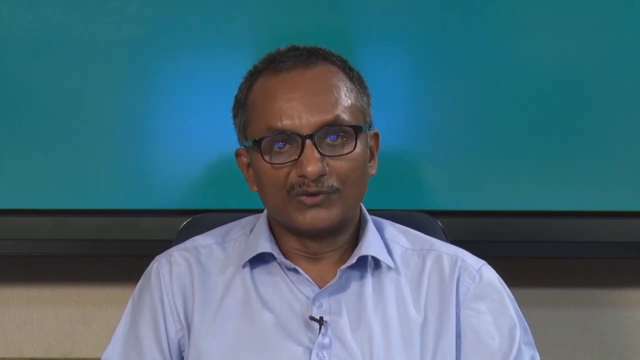 material comes up. I mean, the composite materials is actually is an example of the latter category, that is, it comes under the new material. So why composite materials to come in the quest of improving? So how to do this? So let us first define what exactly is composite? ok, Composite is. 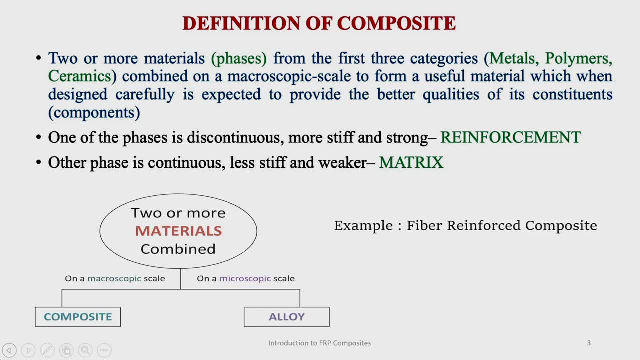 two or more materials, or sometimes is also called phase. So two or more materials are actually taken from the first three categories. I mean we have already categorized the structural materials as four categories: metal, polymers, ceramics and composites. So two or more materials are actually taken from the first three categories. 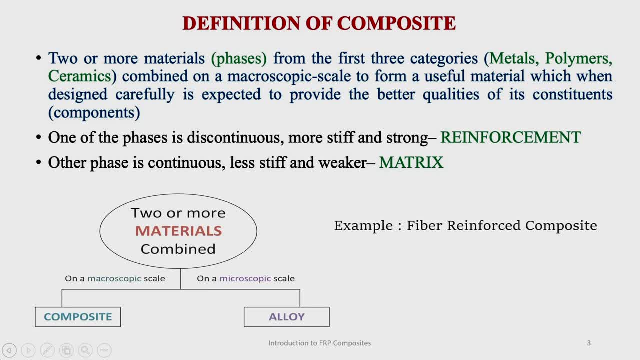 combined on a macroscopic scale. This is important: that they are combined in macroscopic scale to form a useful material which, when designed carefully, is expected to provide a better quality of its constituents. That means two or more materials are mixed and combine macroscopically. 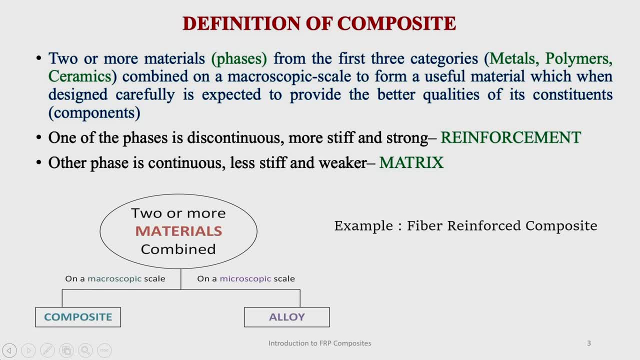 with an objective: that it will give improved performances which none of the constituent materials could provide alone. ok, One of these two phases is discontinuous, more stiff and stronger, and is termed as reinforcement. ok. 5.5mm, 4.6mm, 6.1mm. 7.9mm, 28.2mm, 8.9mm, 29.9mm, 29.7mm phase is continuous, which is less stiff and weaker, which is termed as matrix, naturally say the why it is called reinforcement, because it actually enhances the strength or stiffness. 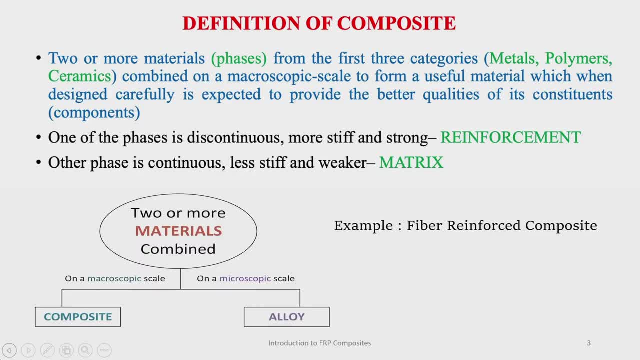 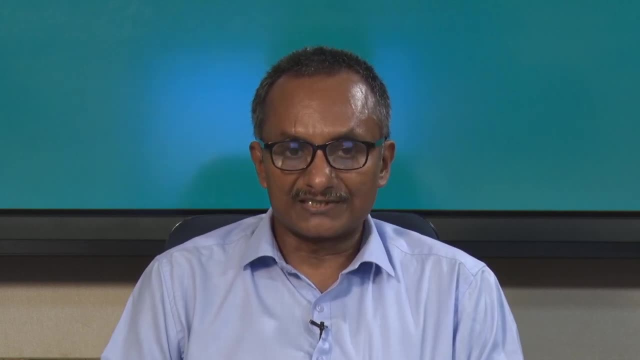 when it is added to another material. therefore, it is a reinforcement, it is a discontinuous phase. So, in so, what is a composite material? now we understand. we understood why a composite material had to be thought of. and a composite material is actually two or more materials. it is shown in this schematic: two or more. 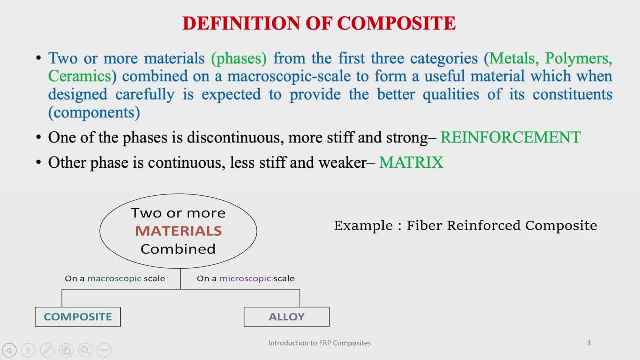 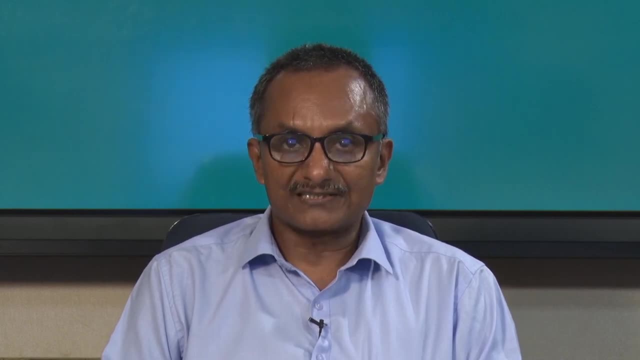 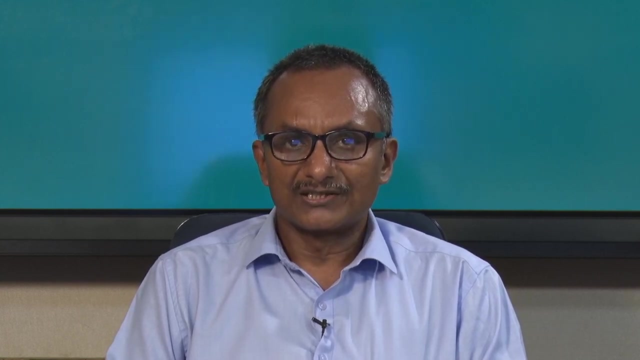 materials combined on a macroscopic scale to have certain desired properties, which is better than the individual constituent components. and this is composite. Now in alloy also we mix two or more materials, say alloy steels. we use number of components to make an alloy. of course they are also. we do it with an objective of getting certain desired properties. 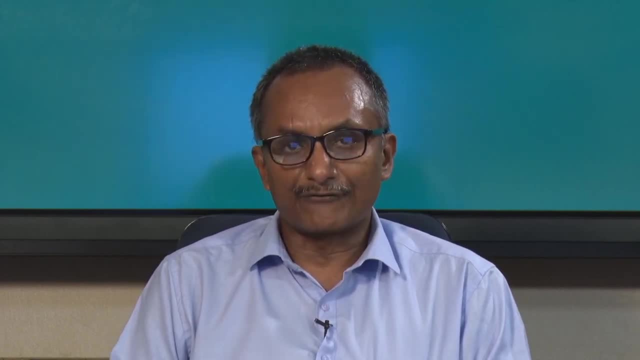 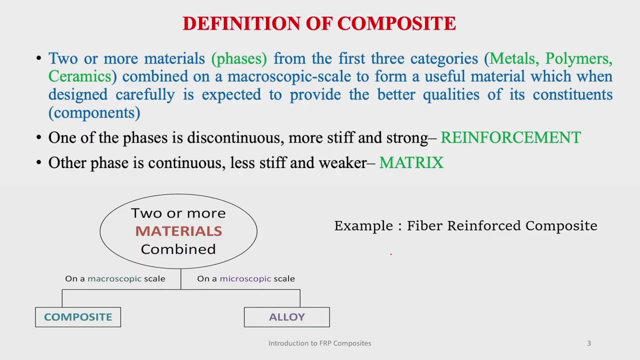 but then they are actually mixed in microscopic scale. therefore they are not termed as composite. ok, This is important. what is macroscopic and what is microscopic? this is important like we can understand this with a simple example. say, for example, if you take a composite, 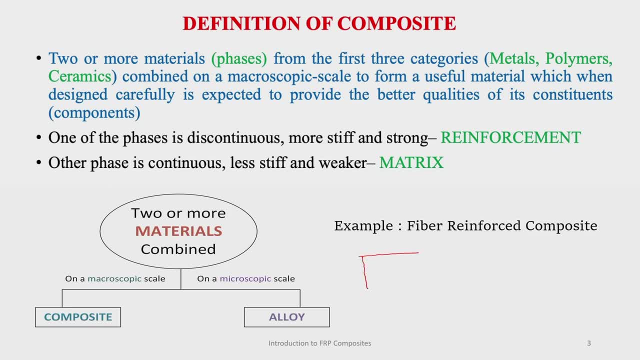 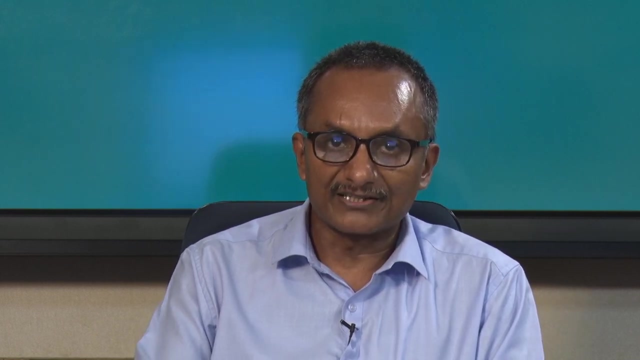 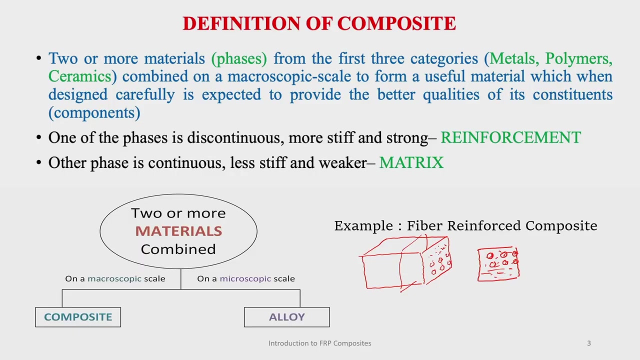 suppose this is a composite, So you can see that the two constituents, one is the reinforcement, which are the rods, and other is the aggregates. So if you take a cross section with naked eye we can actually clearly see the two distinct, you know, must faces. ok, On the other hand, suppose if you 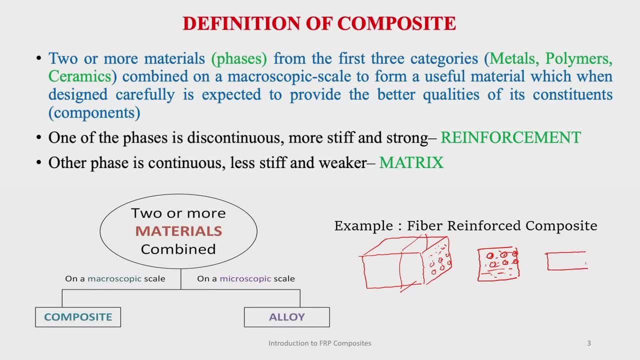 consider an, a bar made of alloy steel. ok, a bar made of alloy steel, and take a cross section. you cannot make out with naked eye that it actually consists of more than one material, even though it consists of i, d n, carbon. you know, manganese may be vanadium, So 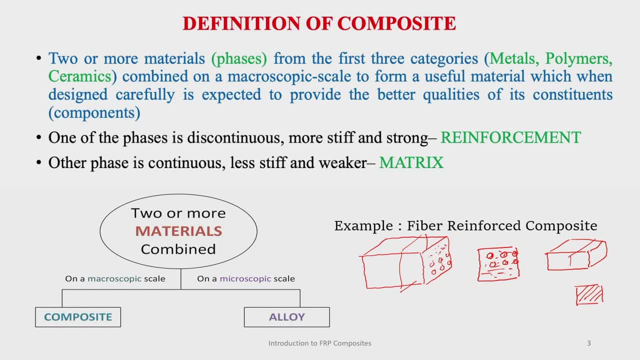 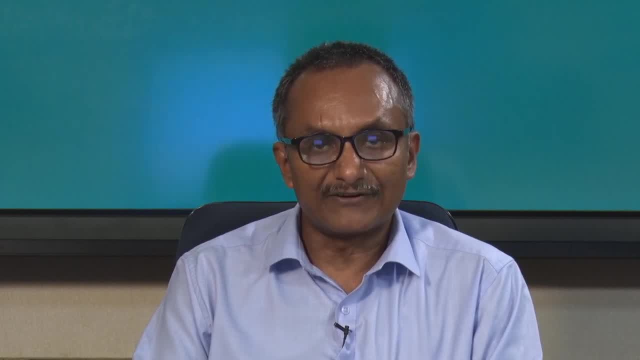 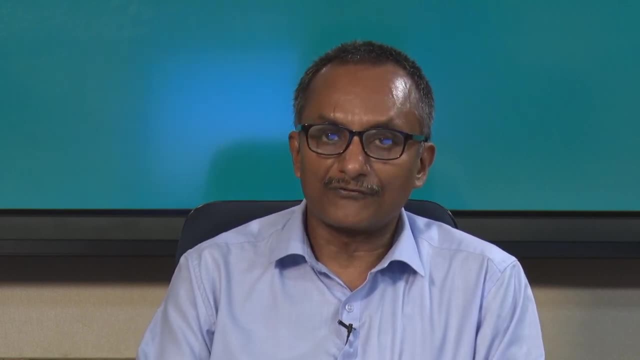 you cannot make out until and unless we actually put it under microscopic microscope and then we can see the district faces different. therefore it is not a composite, the it has to be mixed in the macroscopic scale. So on common example of ah composite is fiber reenforced composite. 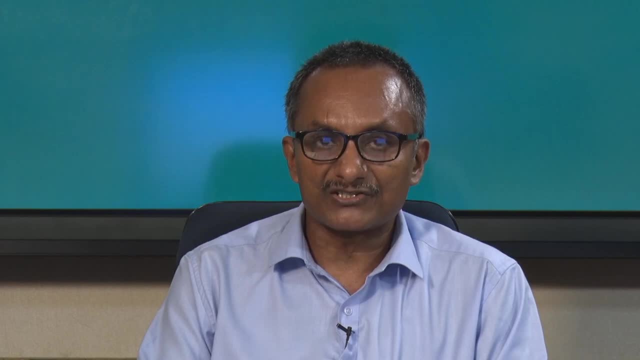 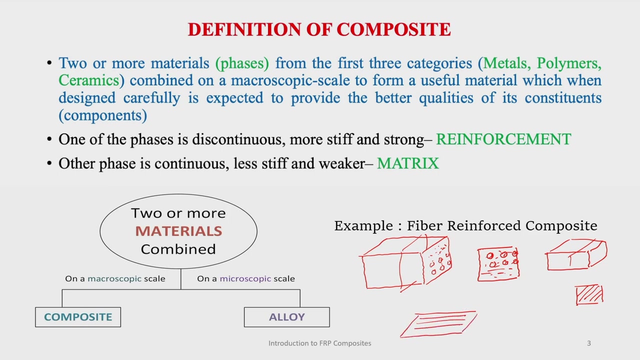 you know the nowadays it is extensively in aerospace applications, where glass or carbon fibers that are actually mixed, mixed with polymeric matrix and they are used as a structural component. So it actually looks like this: there are large number of fibers and they are actually mixed with polymer. 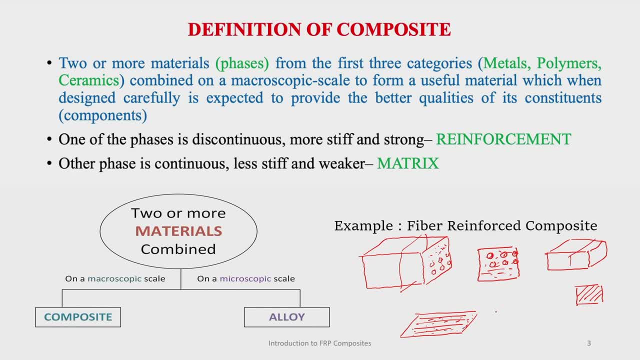 matrix. many a case these are epoxy resins. So the two distinct phases are: the fiber is the reinforcement and the polymer is the matrix. Now, what do you mean by discontinuous and continuous, if you can see? here I mean, I can enlarge this figure little bit, suppose. 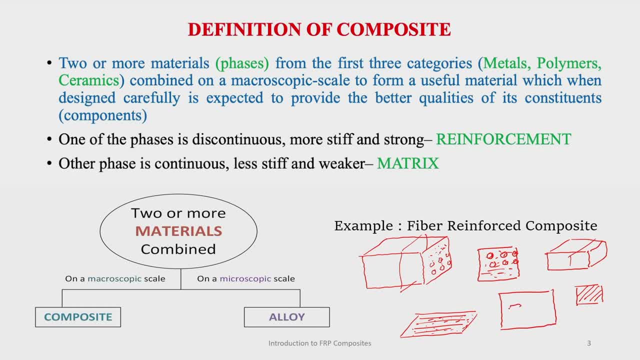 if you look at just only two fibers, say I am drawing just two fibers and rest is matrix. so this fibers are discontinuous phase because you cannot reach from one fiber to another directly. But this matrix is continuous. you can reach from any point on the matrix to another point. 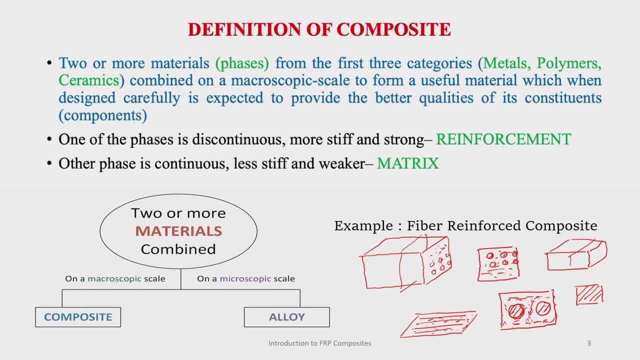 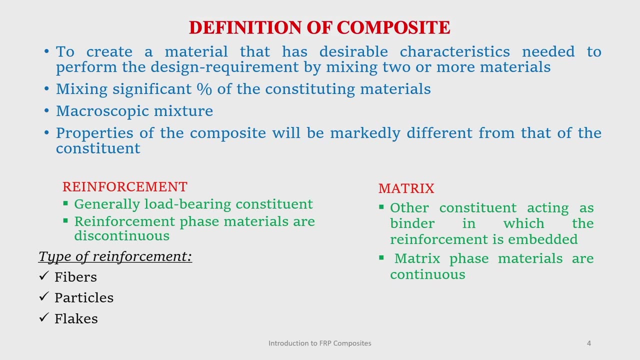 on the matrix. therefore it is a continuous phase. So we could understand what is composite, the basic definition, and we have also seen why an alloy is not termed as composite. this is important to obtain a desirable characteristics and which is needed to perform the design. 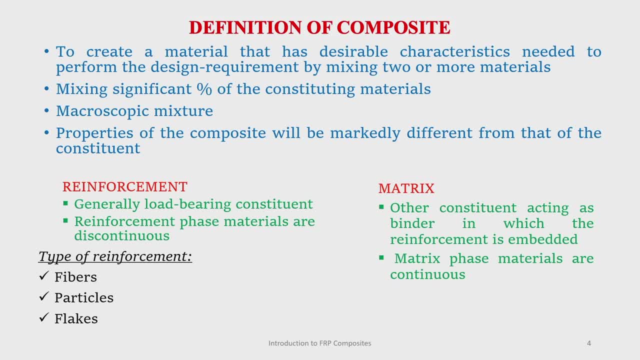 requirement for some functional requirement. Say, for example, we want a component which should be very strong, So at the same time it should be light. Now, as we know that the metals are generally dense compared to, say, polymers, therefore, weight of metals are much more compared to. 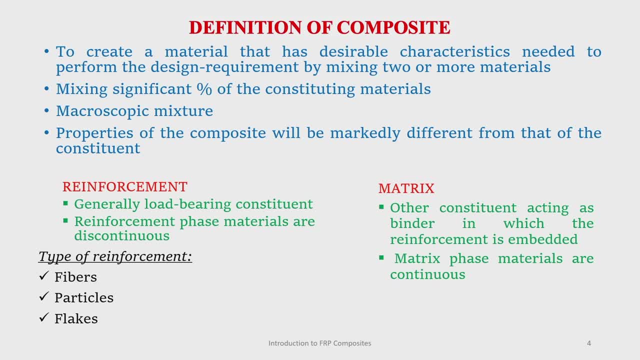 polymers, but at the same time they are far stronger compared to that of polymer. Now could we actually mix, say, a metal, maybe in the fiber form, with a polymer to obtain a material which is strong at the same time light. So this is what we mean by mixing. 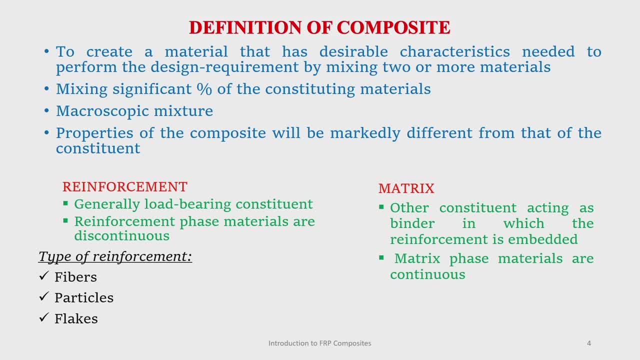 or combining two materials macroscopically to obtain certain desirable characteristics. Second significance is: second point is it should be macroscopic. I have already emphasized that the material should be two. material should be combined in macroscopic scale. That means if you just look at the cross section of the of the composite material, you should. 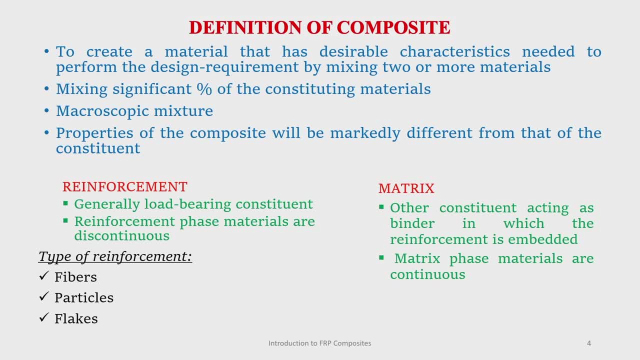 be able to make out the, we should be able to make out the constituents. That means we should be able to, we could see that one is the fiber, other is the matrix, which is not possible, like in alloys, Because they are not actually mixed at macroscopic scale. they are actually mixed or combined. 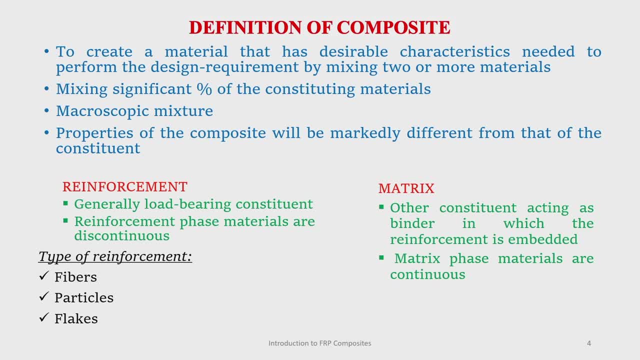 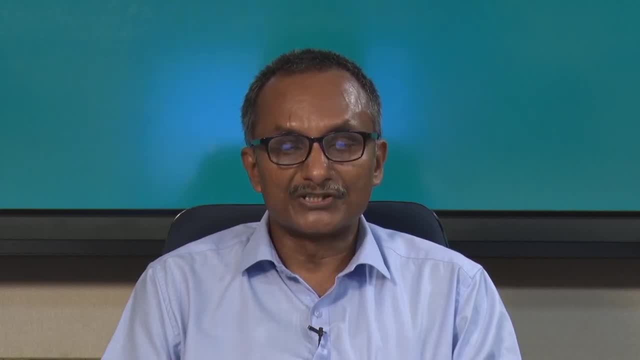 in the atomic or microscopic scale. therefore, it is not possible to identify the constituents using, you know, just by visual inspection, until and unless you actually put it under a electron microscope. Therefore, these are the characteristics of a composite material, And then the properties of the composite will be markedly different from that of its that of the constituents. Say, for example, just now we have discussed. say, for example, suppose the a polymer matrix, a polymer, say, kind of epoxy, is actually reinforced by, say, carbon fiber. So the Young's modulus of polymer matrix is generally in the range of 3 to 5 giga Pascal. 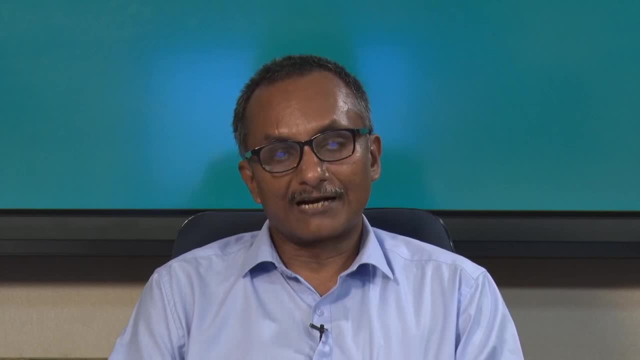 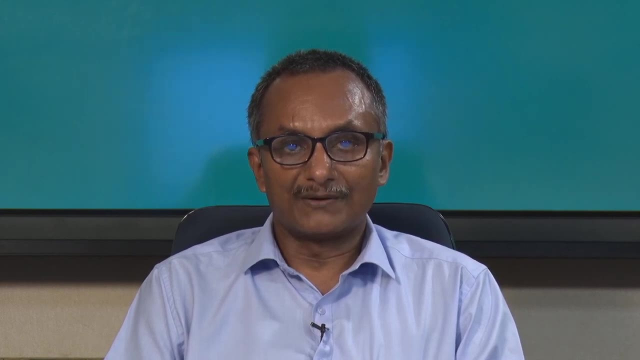 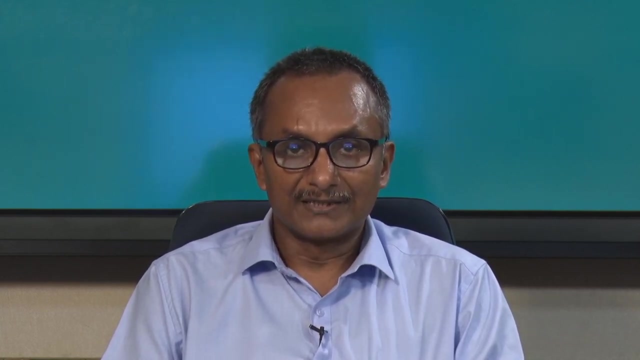 However, for The Young's modulus of, you know, the graphite fiber is of the order of 200 giga Pascal. therefore, if we mix them at a certain you know proportion, say 40 percent graphite and 60 percent polymer, then perhaps the Young's modulus of the, this poly, this composite, this composite will be: 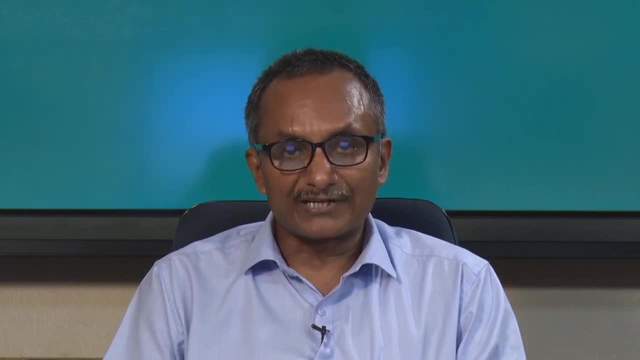 around 180 giga Pascal. So there is a marked difference between the Young's modulus of the, you know Young's modulus of The polymer and that of the final composite. On the other hand, suppose if you talk about an alloy, say addition of carbide in carbide- 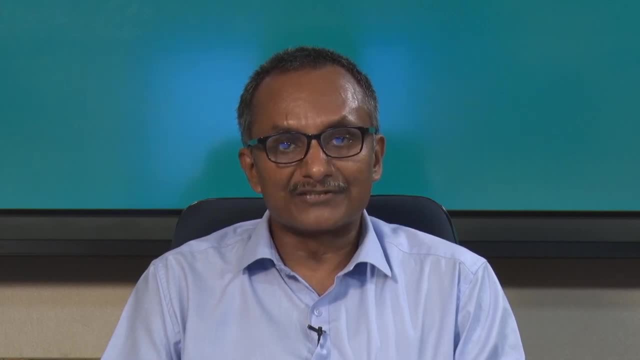 steel hardly has. the influence on the Young's modulus is insignificant. So this is not the case in alloys on the, but in case of composite there is a marked difference in the properties of the final composite, And then there should be significant percentage of the constituent, like suppose, if we talk 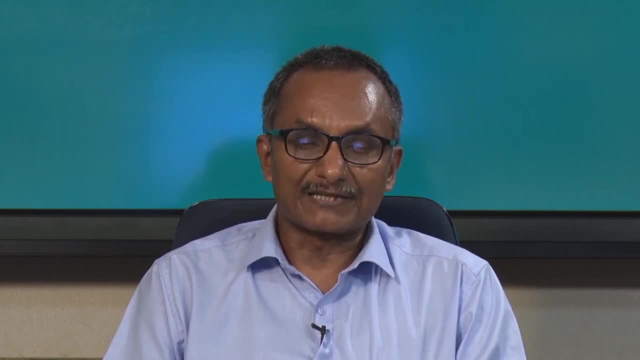 about a polymer matrix, Fiber matrix, Fiber composites, say 40 percent fiber, 60 percent polymer matrix. may be 30 percent fiber, 60 percent polymer matrix, But the percentage is significant, unlike, say, in case of a, say, alloy steel. say there is 0.3 percent carbon, there is, say, 0.04 percent of manganese, like that 0.8 percent of, say. 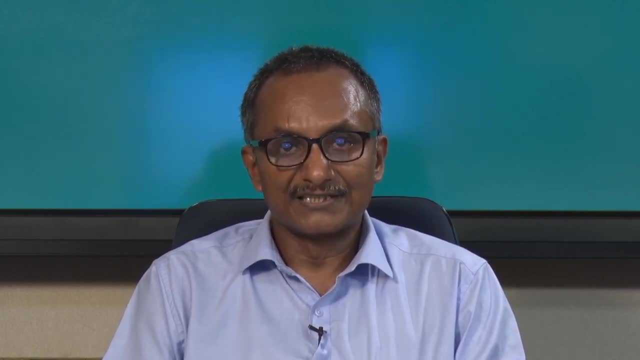 sorry, 0.04 percent of manganese. So the percentage of these elements are insignificant, but on the other hand, in a composite there is a significant percentage of the constituent material. So therefore, to summarize, a composite will have actually a reinforcement phase, which 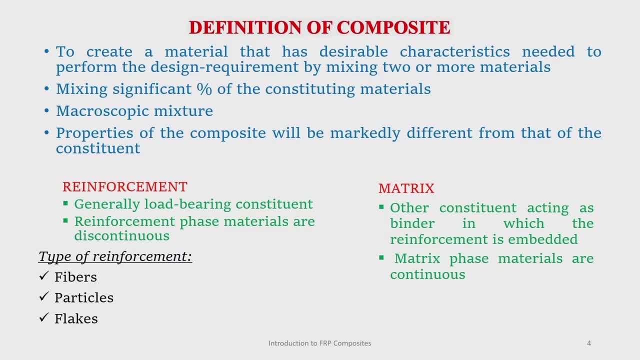 is generally the load bearing, constituents and reinforcement materials are discontinuous. On the other hand, the other phase, the matrix, actually acts as a binder in which the reinforcements are actually embedded and the matrix phase are continuous. So the reinforcement could be of different shapes. it could be fiber, it may not be all. 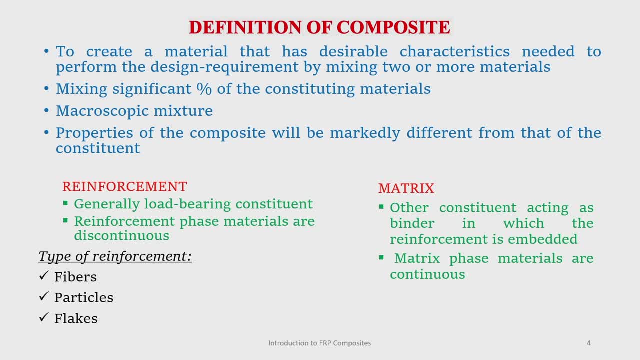 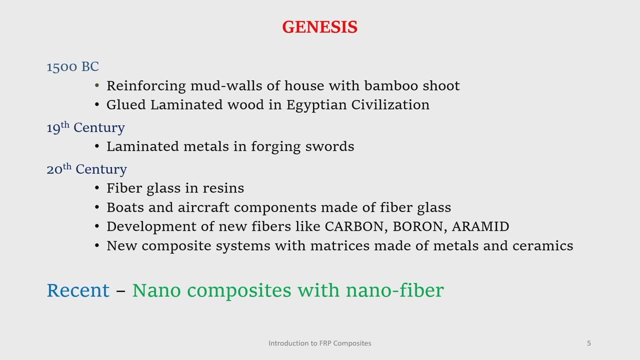 as most of the times we talk about fiber composites, the reinforcement may not be all as fiber. it could be particles, leading to what is known as particulate composite. it could be flake, leading to what is called flake composites. So, having understood the definition of composite, that means when the in the quest of improving. 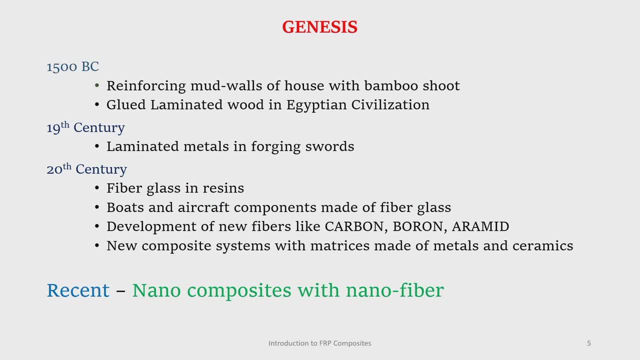 the properties when it was not possible to achieve Achieve that through conventionally available monolithic materials. so in the form of new materials. the composite materials have come up. Now let us see the genesis. are they really new? there have been traces of, you know, reinforcing. 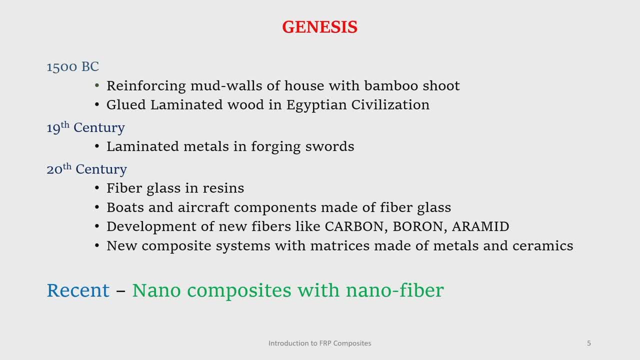 mud walls of house with bamboo shoots. I think even if you now also if you go to villages there are huts, you know where the walls are actually made of mud, where there are bamboo shoots are present. basically, the bamboo shoots are the load bearing member, members and the 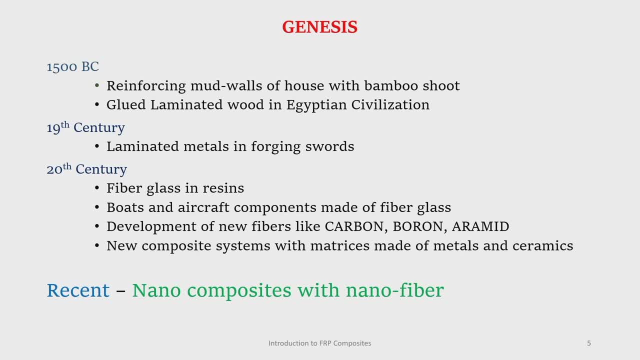 mud actually acts as a binder, Like the bamboo or the reinforcement, and the mud is the matrix, so that this has been there in BC before it is that traces have been there in BC and in the 19th and century. there are examples of, you know, traces of laminated shots used in wire, made of laminated metals by forging. 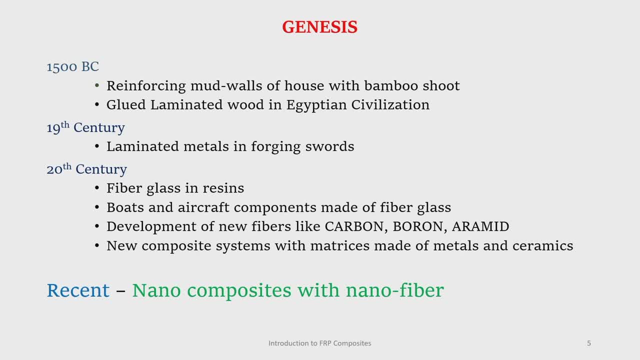 Then in the 20th century, in the mid of the 20th century, first the fiberglass in resins are used For structural components. boats and aircraft components are made of fiberglass. then in the later part of the 20th century, actually the development of new fibers, modern fibers. 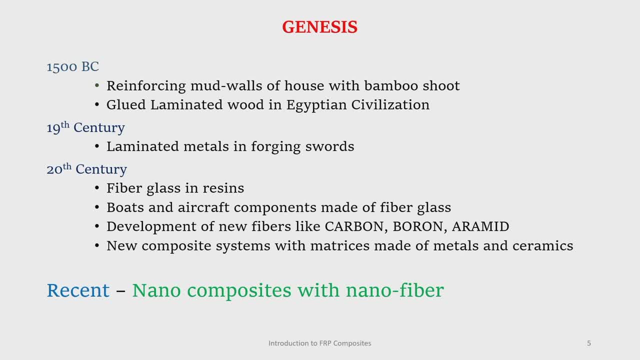 like carbon fibers, boron fibers, aramid fibers, have come up Then new composite systems with matrices made of metal as well as ceramics have been used in in the later part of 20th century, leading to what is known as metal matrix composites and ceramic matrix composites. 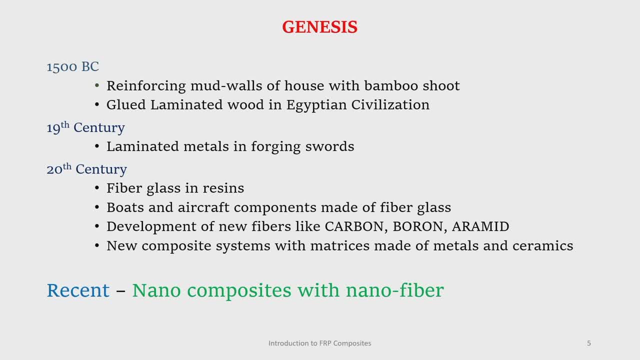 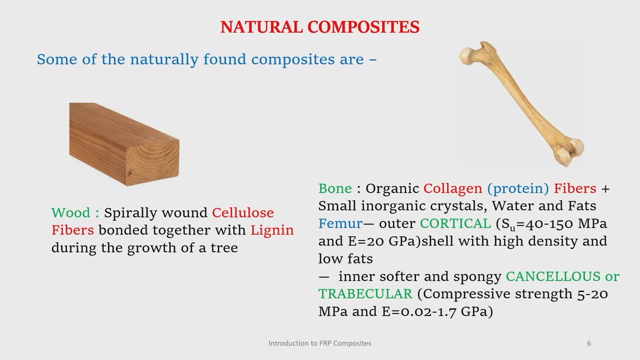 Very recently. there are nano composites where the nano fibers are used. again, the requirement is the nano fibers have much, are much stronger and stiffer compared to, again, so called conventional fibers. therefore, they provide much better strength and stiffness to the composites. In addition, there have been number of examples of natural- you know, naturally- available composites. 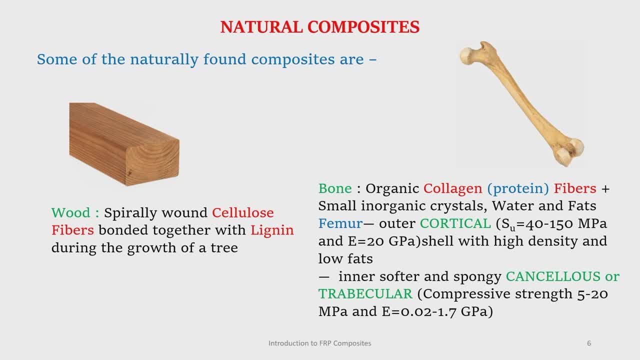 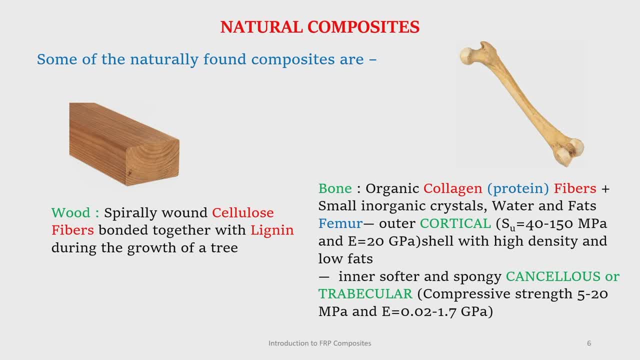 fibers, which is made of protein and small inorganic crystals, water and fats. So, for example, if you look at the femur of a human femur, the outer cortical part- outer one is the cortical- which is having a strength of the order of ultimate strength of 40 to. 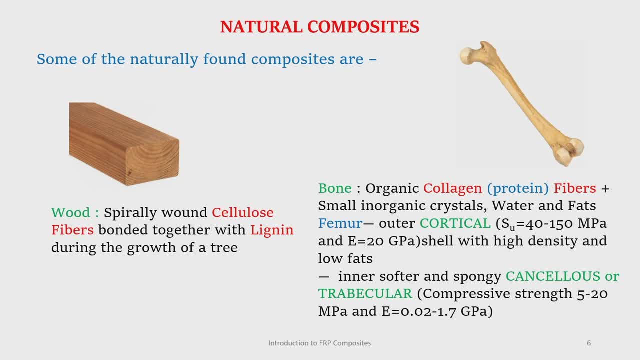 150 mega Pascal with a Young's modulus of 20 giga Pascal. Inside this there is a softer spongy cancellous or trabecular with a compressive strength of around 5 to 20 mega Pascal and Young's modulus in the range of 0.02 to 1.7 giga Pascal. 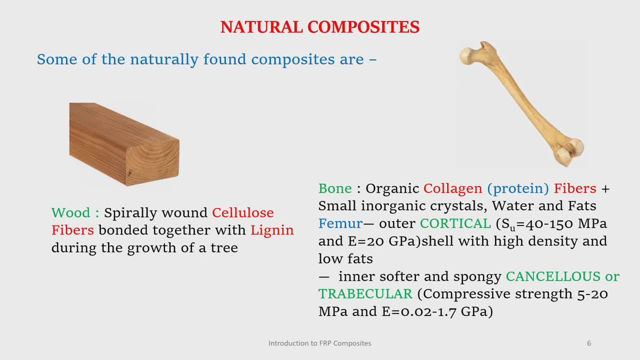 that is much softer. So naturally available composites are there, and these are, of course, with certain objectives. why this is like this? because it has to take a typical kind of load, you know. So again, there is, say, an example: is wood? if you take the cross section of a tree, you 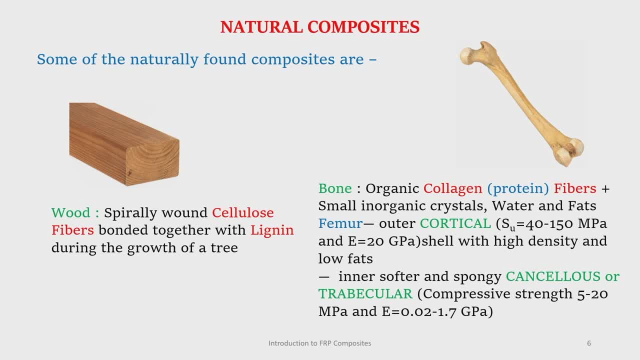 can see the spirally owned cellulose fibres bonded together with lignin matrix. this is formed during the growth of the tree and you know the directional strength of the wood. you know. So because of this, because it is a composite material, they are having direction dependent. 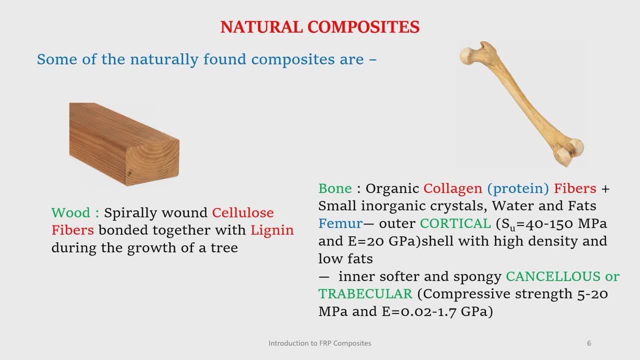 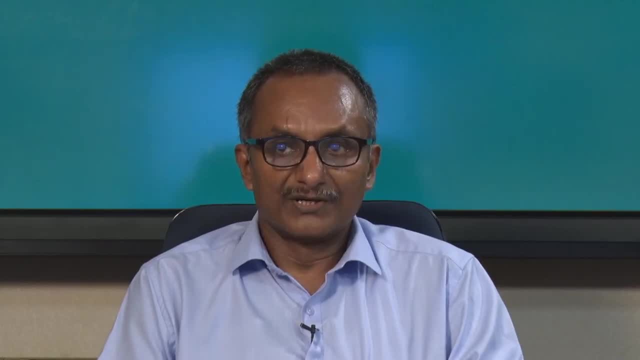 strength and stiffnesses. So even though composite material, the idea of composite material- has been new. may be it has started from 20th century, But it has been, It has been there. I mean, the composite materials have been there much longer. the traces have. 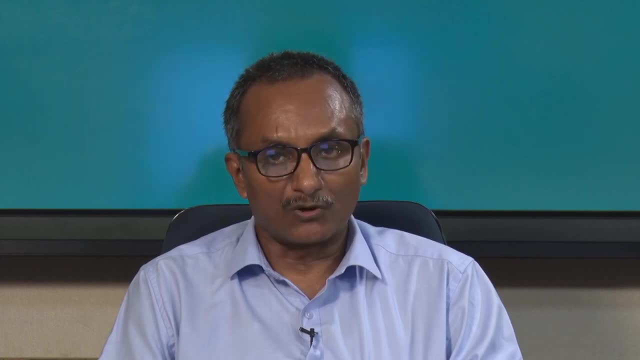 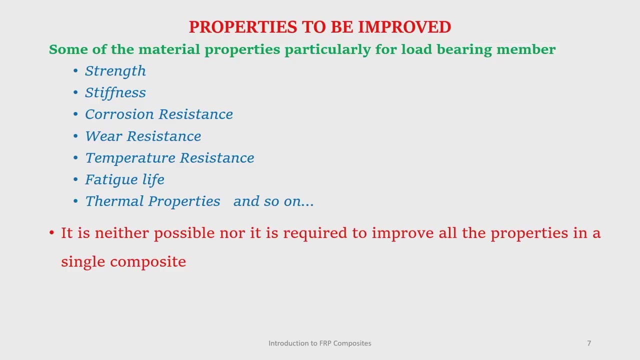 been there even in BC, and there are naturally available composites also. Now in the definition we discussed that two or more materials are actually combined microscopically in order to have certain improved qualities or properties. Now what are those improved properties, say, from the structural point of view for load? 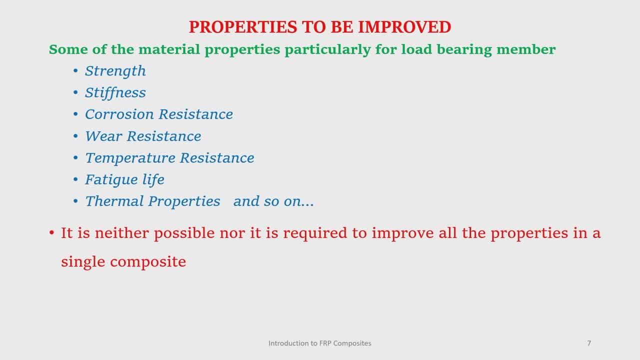 bearing member So many a times. we want the strength to be very high. we want the component to be stronger- may be it has to withstand a very high load. Then we want this to be stiffer so that we may need to improve the stiffness. 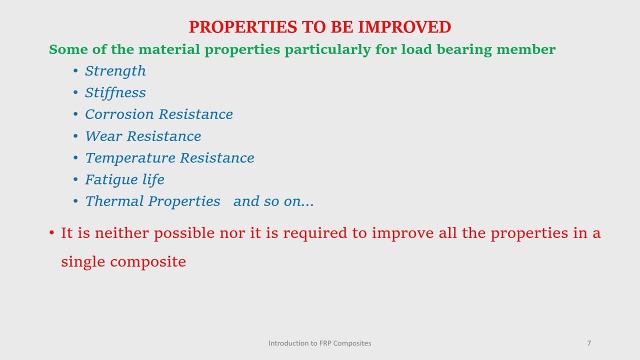 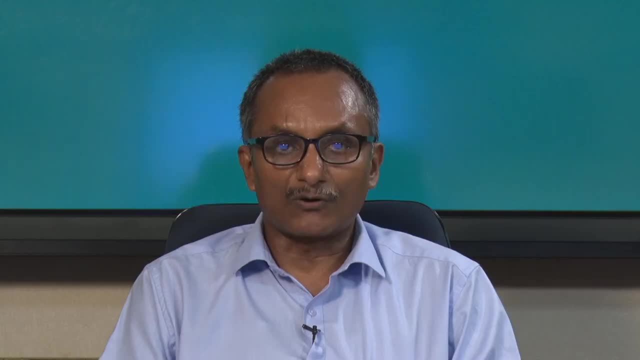 Then, depending upon if a particular component is actually in a corrosive environment, it must have adequate corrosive resistance. then in case of components which are intimate contact, say for gear teeth, So wear resistance is also there, So we can say that these components are very much resistant. 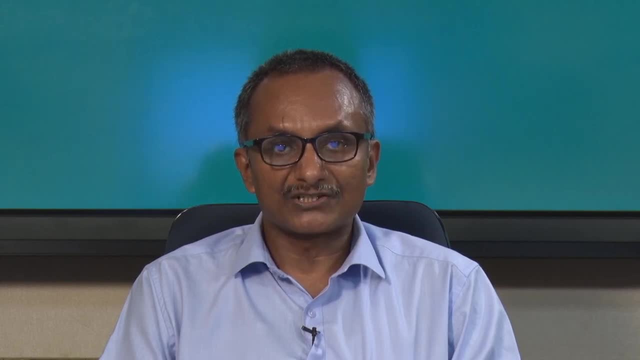 also important. Then there are high temperature applications, where we want the component to be, or the material to having a very high resistance to temperature. Then many of the many structural components are actually subjected to fluctuating load and stress and therefore it is important that their fatigue life is improved. Similarly, thermal properties like coefficient 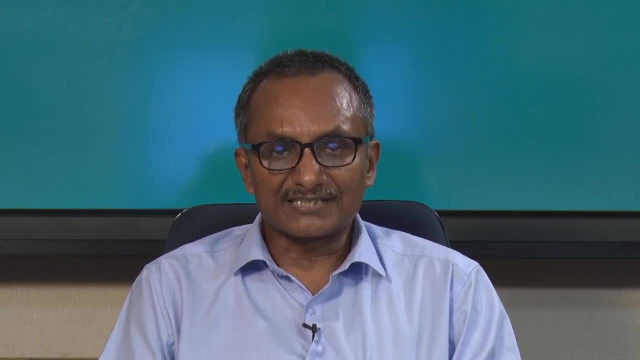 thermal expansion, thermal conductivity. So there are many such properties which needs to be improved. but make sure that it is not possible to increase all the properties in a single composite and, more importantly, neither it is required- It is not required for a particular 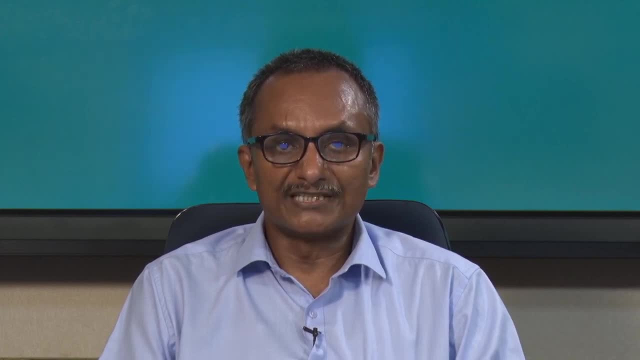 application. we may need one or two or three properties which needs to be enhanced and accordingly we decide what should be the composite material. For some other applications we may decide for a certain specific- I mean properties. we may go for design of a different, I mean look for a different component. 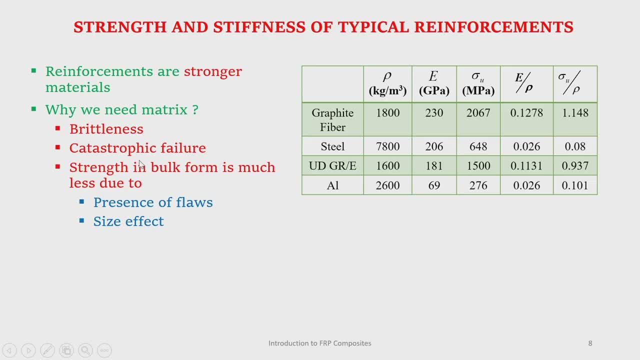 Now let us talk about some of the typical reinforcements. Say there are, as we have discussed, that there are, different types of reinforcement. it could be fibers, it could be particles, So say, for example, in this table we have shown, say, graphite fiber. So, as we have understood, 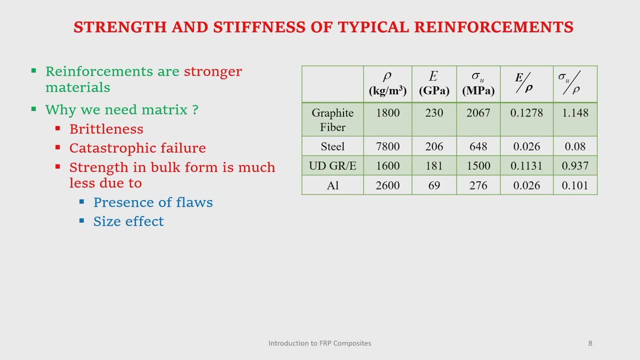 that the reinforcements are far stronger and stiffer- I mean usually- compared to the matrix, Say, for example, in this table. if you look at the graphite fiber, say, for example, in this table, if you look at it, the graphite fibers has a Young's modulus of 230 gigapascal. 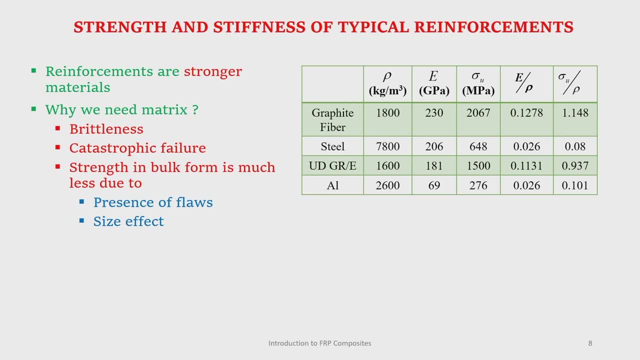 and if you compare this with steel, which is having a Young's modulus of the of the order of 200 gigapascal, So they are more or less I mean same order they, while the Young's modulus of the graphite fiber and the steel is almost same. but if you look at the strength, 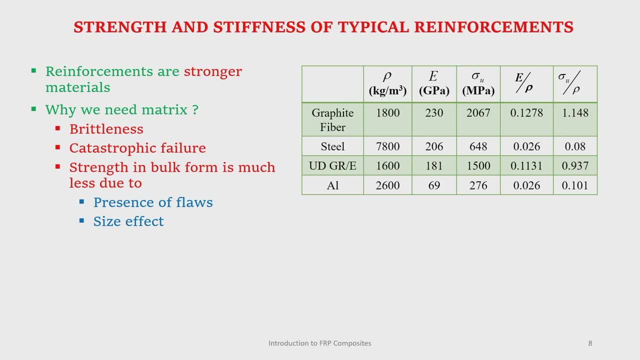 ultimate tensile strength of graphite fiber is almost, you know, three times that of the steel. So if you look at this table, the strength of graphite fiber is 2000 mega Pascal, whereas that of a typical steel is 640 mega Pascal. so it is almost three times. so it is three. 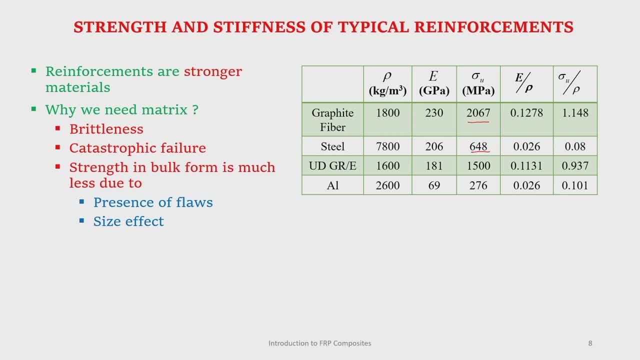 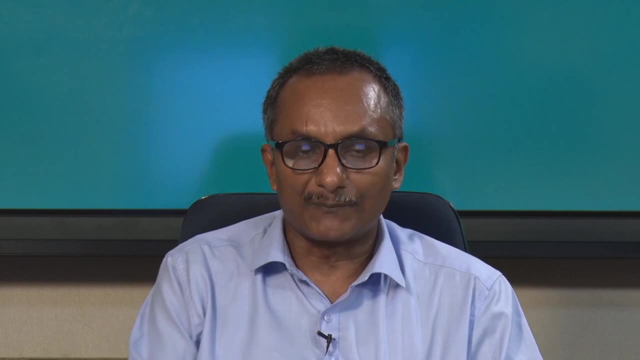 times stronger. Similarly, this shows unidirectional graphite epoxy we will have. we will discuss this in detail. so, when we come to the fiber reinforced composite- but here what it means is graphite fibers are actually mixed with polymer matrix to give graphite epoxy, so this is the composite. 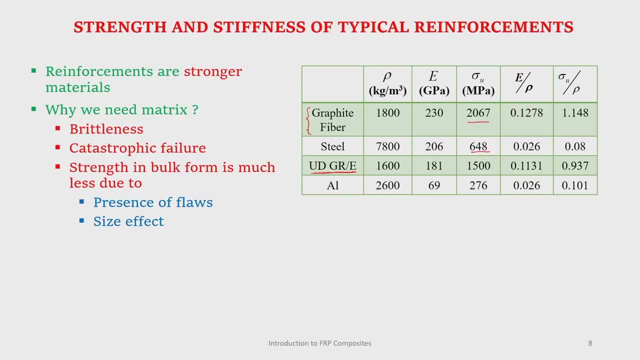 actually this is only the reinforcement and this is the composite. so at a certain percentage the graphite fibers are mixed with polymer composites and that also gives to, gives rise to a Young's modulus which is comparable to that of steel: 180 giga Pascal, but strength. 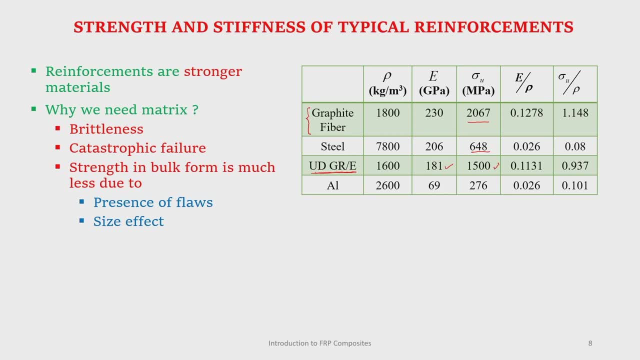 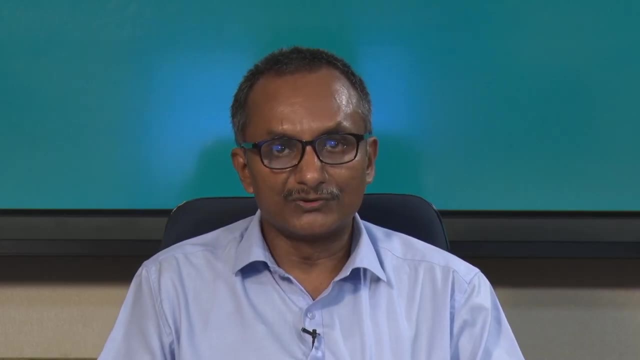 is almost 2.5 times that of steel, so it is still much stronger. Now the natural question comes: if the reinforcement- like the graphite fiber in this case- is such it is so strong, It is so strong and stiff, then why it has to be mixed with matrix we can use, we can. 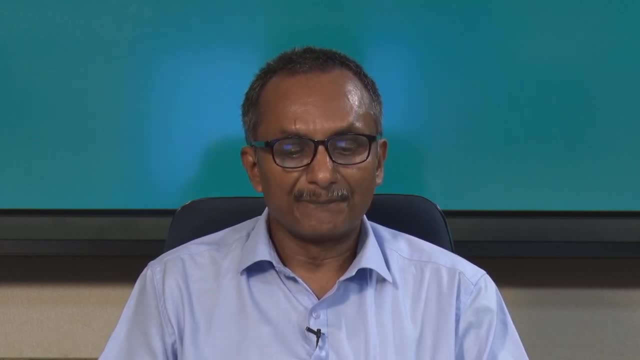 use this material in the bulk form. but this is not done, because most of these reinforcements are actually in bulk form, are not that strong, you know, and they are. mostly they are brittle and leading to catastrophic failure. that means they fail without any warning. but, more importantly, 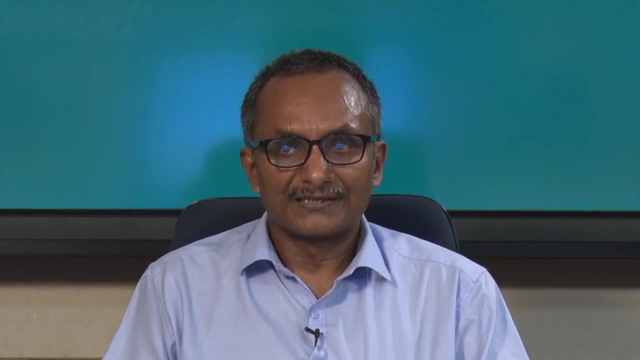 if you take, say, a glass fiber, Okay, It has a certain ultimate strength, but if you take a glass panel, the strength of the glass panel will be much, much lower compared to the glass fiber. the reason is the materials in the bulk form are much weaker. because of the presence of flaws, there will be inherent 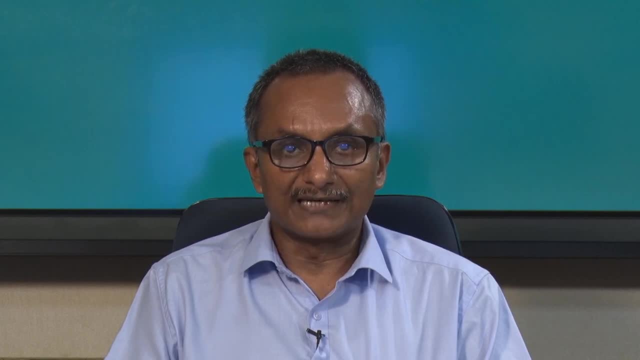 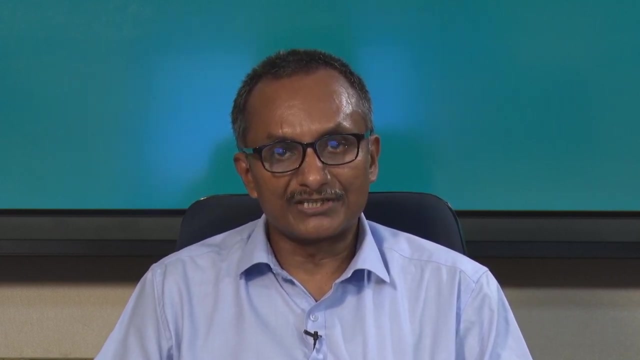 flaws. I think that all of you have done that Griffith's theory, if you have done in material science, Okay, The presence of a flaws actually reduce the, reduces the strength. Okay, So the material in this bulk form will will have more chances of having flaws in it. second, 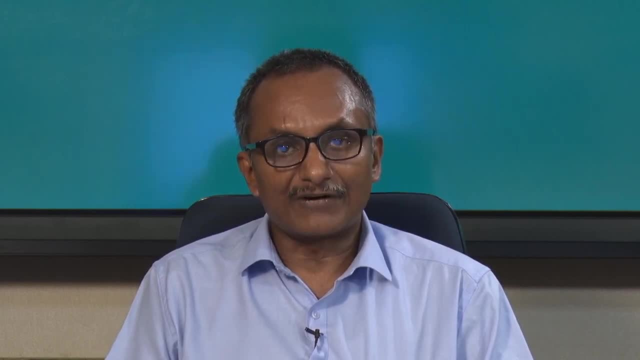 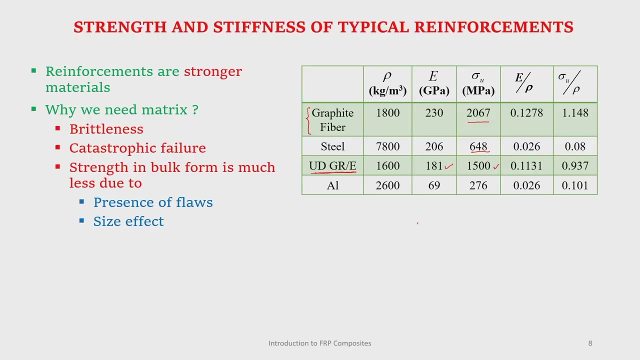 thing is that in its fiber form, because the fiber dimensions is of the order of, in the order of microns, even if there are flaws, the size of the flaw will be much less compared to the flaws in the, you know, in the bulk form. so there is which is called size effect. actually, 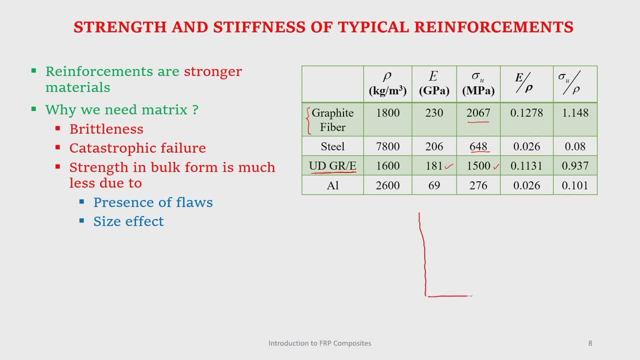 in size effect. So, if you see, this is the size of the flaw, flaw size and this is the strength. it is something like this not to scale. so as the flaw size, you know, increases, the strength actually decreases. so this is why actually it this: fibers which are very, very strong and stiff are actually 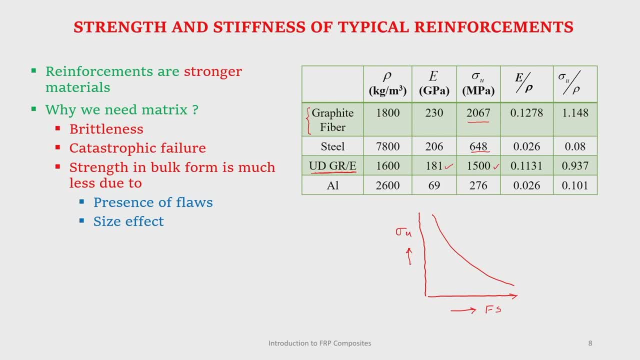 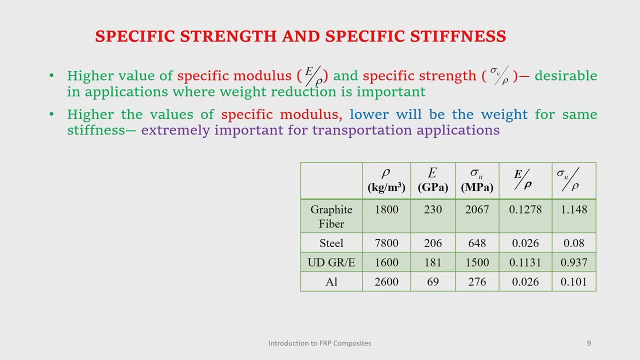 mixed with the fibers alone cannot make a you know structural component. You know structural component and they are mixed with the matrix to make the composites. Now, another important thing is if you notice in this table that even though the Young's modulus of graphite fiber or, for say example, the Young's modulus of the composite graphite, 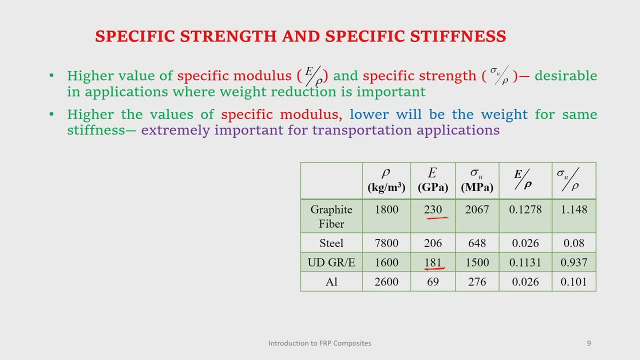 epoxy composites. that means graphite fibers mixed with, you know, polymer matrix- that the Young's modulus of the steel, and this is almost comparable. but then if you look at the density, the density of graphite fiber is actually almost four times more than four times less than that of steel and the density of the graphite epoxy composites. that means 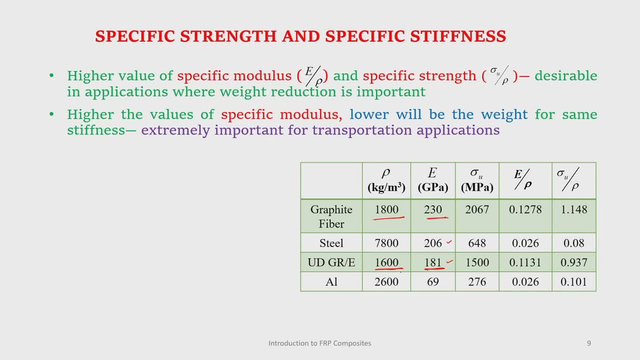 polymer matrix composite with graphite fibers is also much less, you know, almost four point, six times less times that of the steel. This leads to that that we define. this leads to the definition of, you know, specific modulus. What is specific? modulus E by rho, that is Young's modulus. 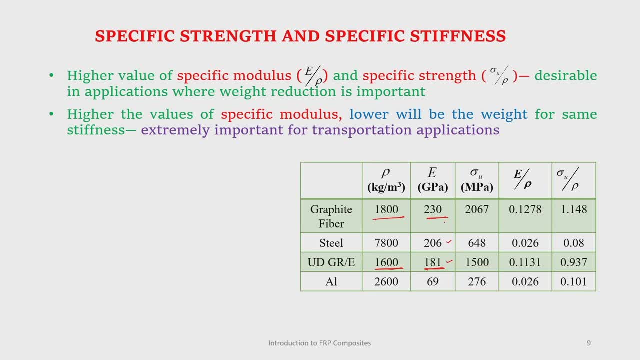 divided by density. So if you see that, even though the Young's modulus of the steel and this composite is almost comparable, but the specific modulus of the graphite epoxy is almost, you know, 5 times more than that of the steel. Similarly, if you look at the strength, the strength of this composite is anyway, almost 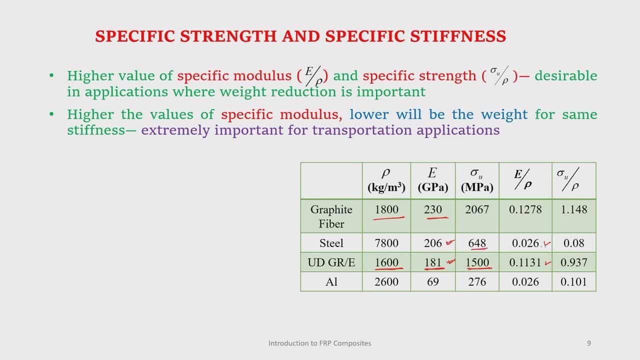 2.5 times that of steel and, when it comes to specific strength, is almost roughly 10 times that of the steel. Now what does it mean? It translates to higher the values of specific modulus. Lower will be the weight for the same stiffness. 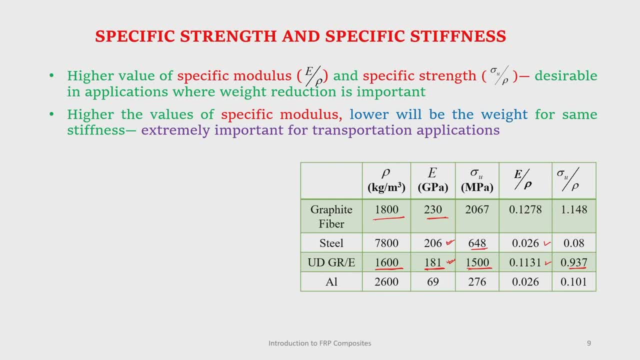 That means, suppose we have two components, one is made of steel, another is made of graphite epoxy, Then they are. I mean, if we want to have the same stiffness in both of them, then what will happen is the weight of the graphite epoxy will be almost 5 times less than that. 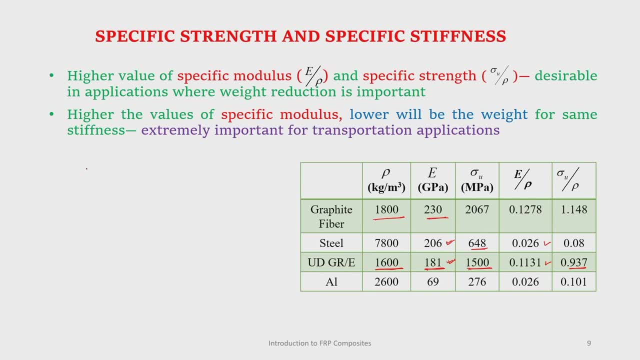 of the steel. Say, for example: we can take this example here, what this. suppose we have one slip back to say bar and say it is. you have, taking a most simple example, a bar subjected to axial load B. suppose the length of the bar is L. uniform cross section, suppose uniform. 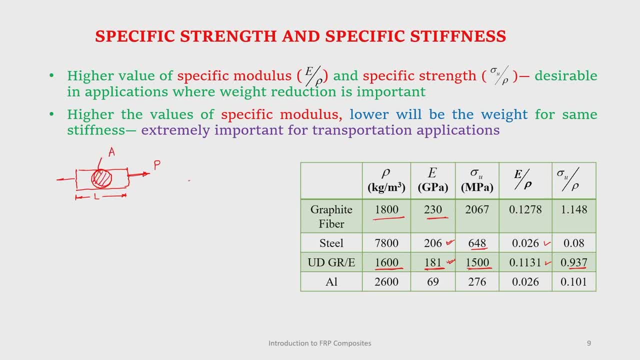 cross section. say the area of cross section is A, we know that the deflection under axial load is pl by Ae. So that gives rise to dated actual放 v. So we can write this: as delta is equal to P, L, square A into L into E, Now A into L. 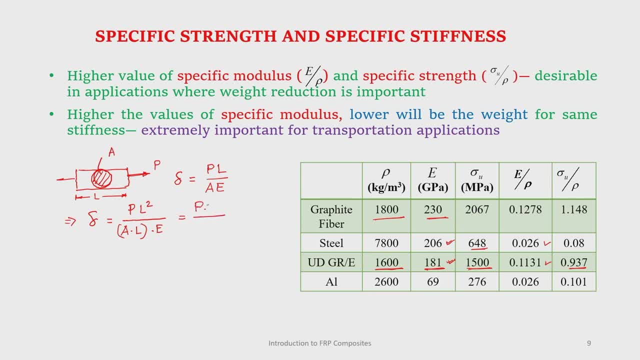 is nothing but the volume of the bar. therefore, this is P L square V. If m is the mass and rho is the density of the material of the bar, then this is m by rho. we can write the volume into E. therefore we can write: delta is equal to P? L square by m into E by rho. 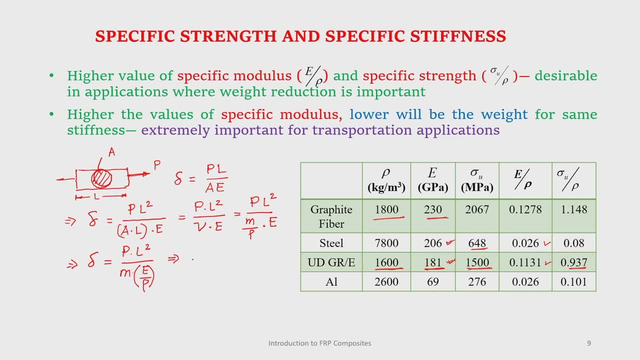 This E by rho is nothing but the specific modulus. therefore we can write mass m into L is equal to P, L square by delta. therefore, if E by rho is twice suppose, then mass will be half for the same stiffness for the same deflection. Therefore, as E by rho increases, 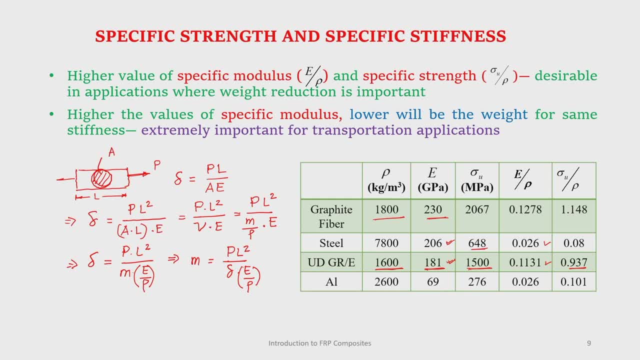 the mass decreases. it has a tremendous implication, especially in the transport sector. you know in where it is used. in the transport sector Say, for example, say, in an aircraft, in aerospace, in an. in an aircraft say, typically the mass of, say, a big aircraft like a, like airbus A320, is around 40000 kg, Suppose in an aircraft. 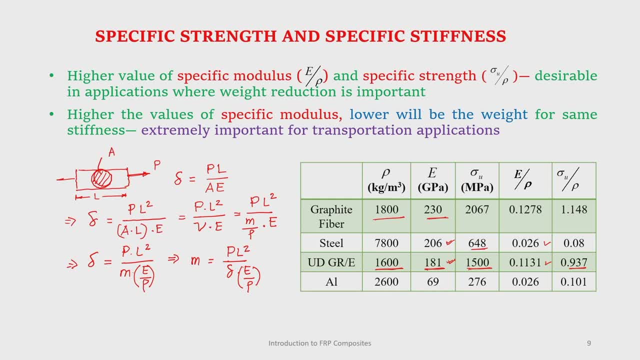 by some means, by using, by changing the materials, if you can reduce the mass by 10 percent, reduce the weight by 10 percent. I mean it is not that easy. but say just, I am giving an example. suppose the mass is 40000 kg. By choosing some lighter materials. if you make it say, reduce the mass by 10 percent, say 4000, that means what happens is this 4000 is the gain in the payload. that means, since you have reduced the mass by 4000 kg, you can actually add 4000 kg more in the aircraft. So it has. 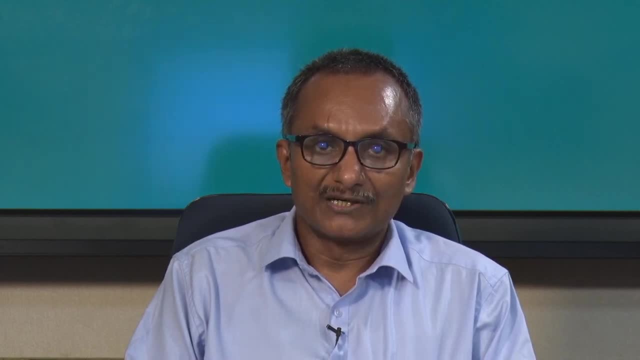 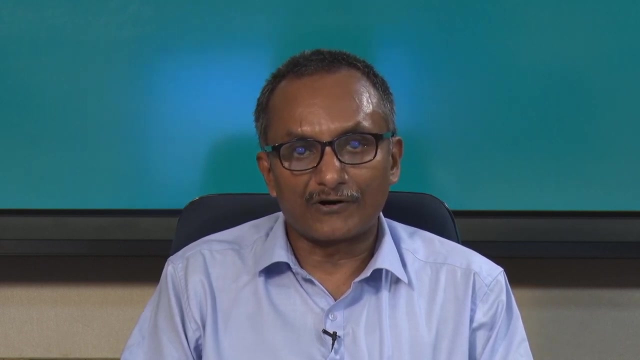 a tremendous economic implication, as fuel savings and you know say, for example, that means you can actually put 4000 kg of different materials in the aircraft and and, and that if the payload is actually increased by 4000 kg, So it has a tremendous economic implication. So same is true for, even for- I mean the launching- 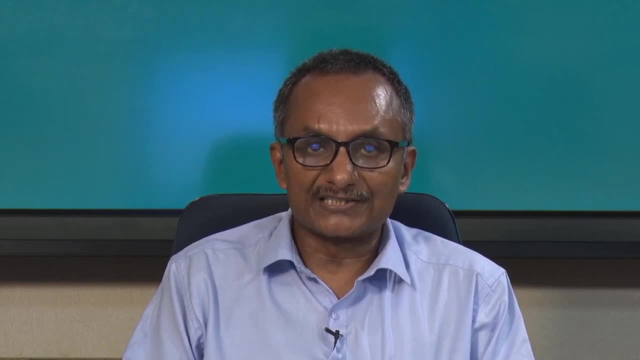 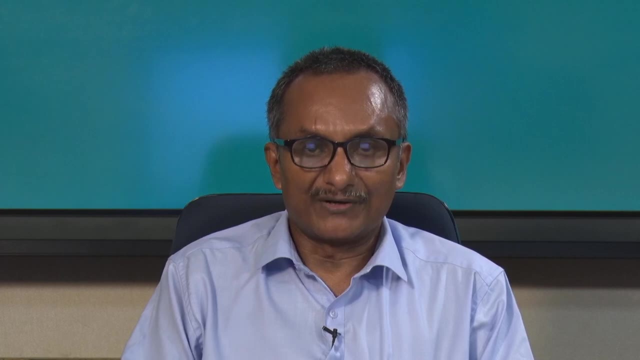 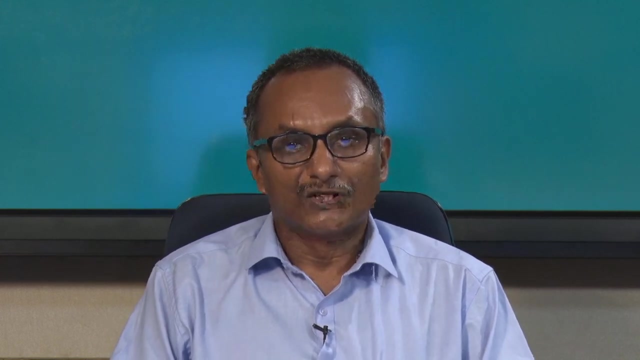 the satellites rocket. ok, If the, if the payload could be increased. that means that is the savings in the. you know that is direct savings in the in the economy, ok, of the whole program. So this is what is exactly the implication of higher specific modulus. therefore, in I 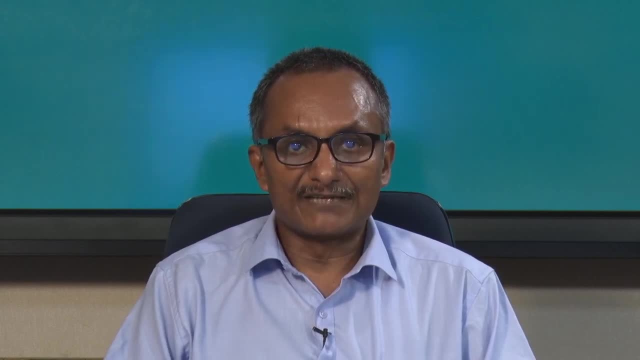 mean is made with the specific modulus, not with the modulus in case of composites. the higher the specific modulus, the lighter will be the material. Similarly the specific strength: the higher the specific strength for the same strength, lighter will be the component. Now it may not be always E by rho. I have just taken an example of axial loading. there it 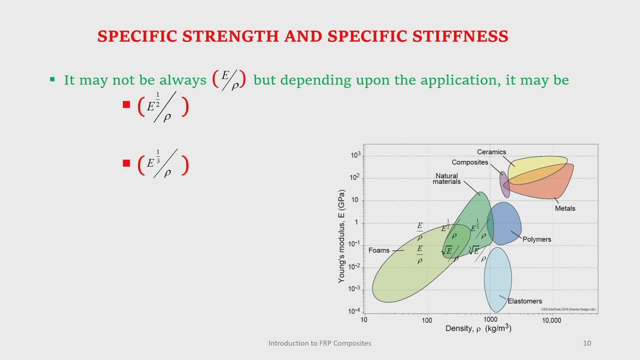 is E by rho, but it say, for example, in case of buckling it is actually root E by rho, because in buckling it is the critical buckling load which actually decides that what is the limiting condition. and from there I am not showing it here. we can show that if E to the power, 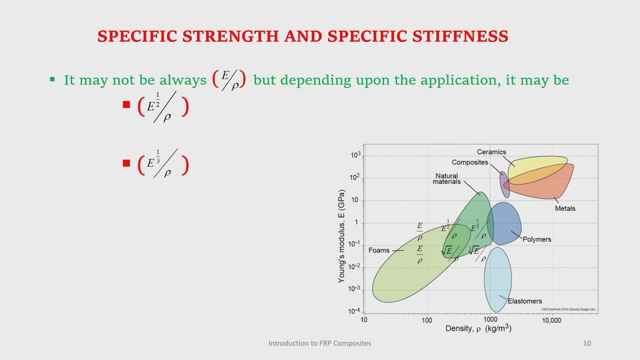 half by rho is maximum. that will lead to minimizing the mass. Similarly, if you take a panel, this is for buckling. Similarly, if you take a panel, this is for buckling. Similarly, if you take a panel subjected to transverse load, a plate subjected to say: 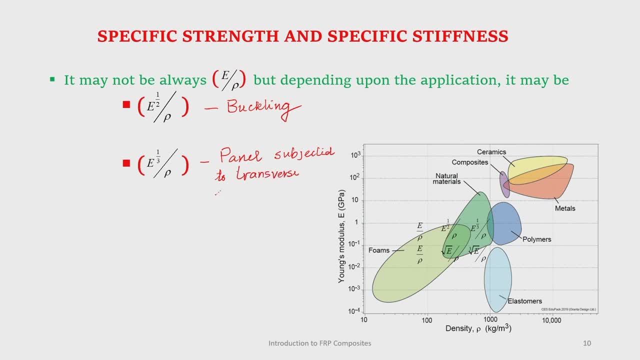 transverse load. So it is actually cube root of E by rho which decides that for the same deflection the mass will be minimum. So all of you might have studied in machine design. I have just repeating it here. this, as by plot you know, this is this side is density and 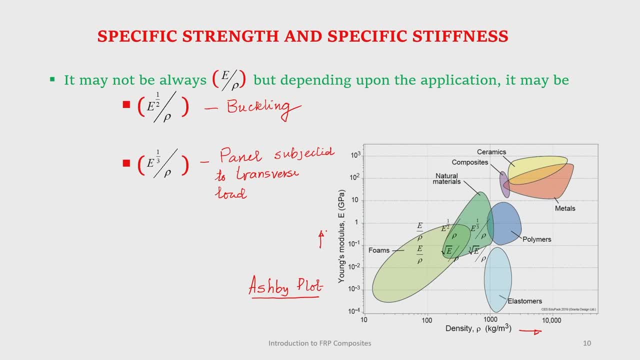 this side is young's, modulus, and you can see different types of materials, right from very load density to very low strength, to high density, high strength. So metals figure somewhere. here you can see the composite. as far as the strength goes, it is almost in the same. 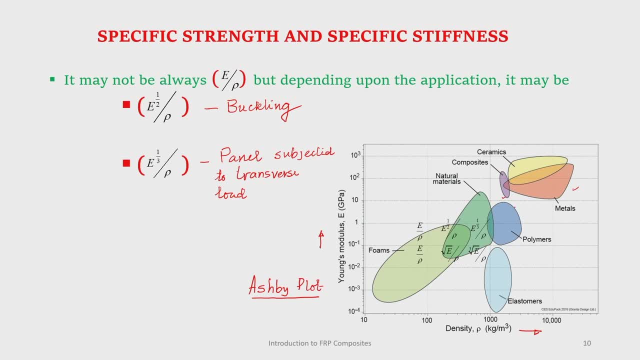 Same place with metals, but the density is much lower in the scale. Similarly, the ceramics say polymer is in between. So this plot is very, very useful in selecting the material. We can find out for a given E by rho. we can have a constant E by rho line here may be: 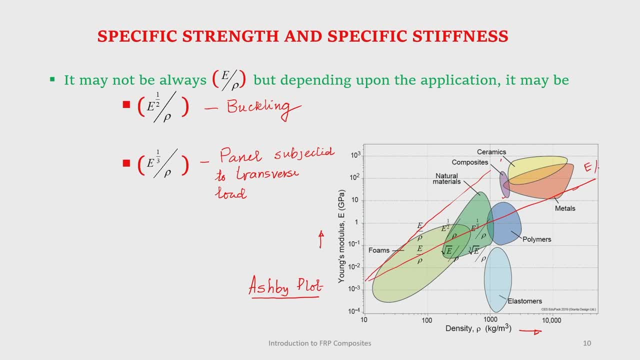 you can have a constant E by rho line here. We can have a constant root E by rho line here and decide what material to be selected based on the functional requirement. So now, having understood the definition of composite, all these what we have been doing, 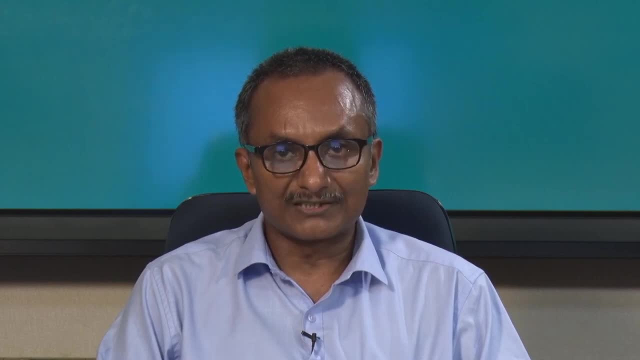 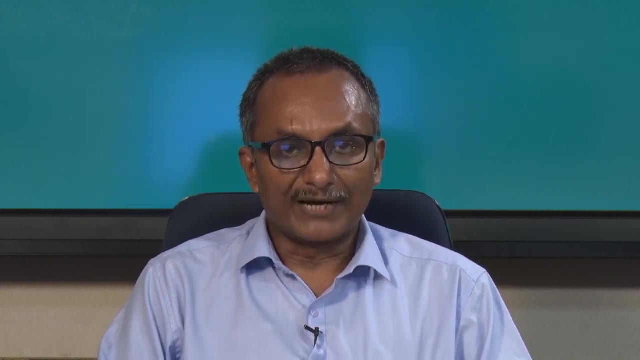 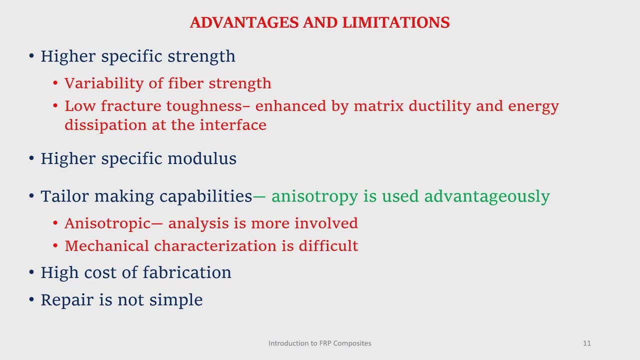 was to understand the definition of composite. what exactly is composite when we say composition, what we actually achieve through a composites? Now there are advantages and limitations also. Now advantage: already we have discussed: it has higher specific strength. why it has higher specific strength? because the reinforcements are far stronger, say, for example, in a fibres. 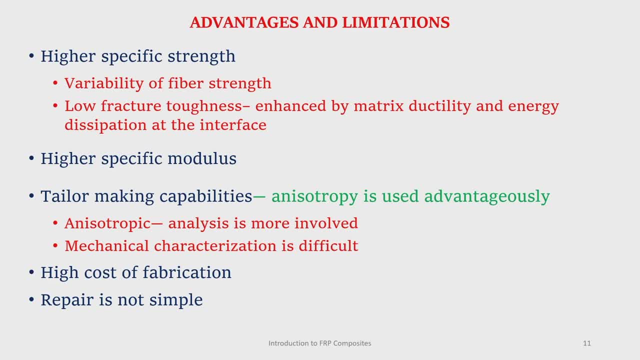 fibres. in a fibre composites the fibres are far stronger, But because of the strength they are stronger. the strength of fibres are actually, the variability is much more compared to the conventional materials. So, and because of the variability of fibre strength, so the 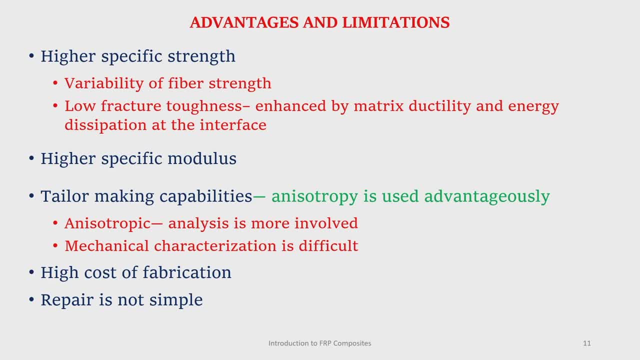 overall strength. variability is more, So that is a disadvantage. and low fracture toughness. the fibres actually behave like brittle material and therefore they have low fracture toughness. but when it is mixed with matrix, like polymer matrix, the ductility of the matrix actually enhances. 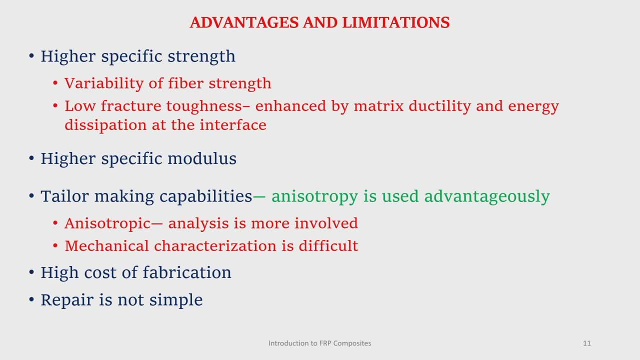 of fracture toughness, sometimes by dissipation of energy. Then it has higher specific modulus that we have just discussed. that means E by rho is far higher compared to conventional material materials. that leads to weight savings in the applications where weight minimization is very important. 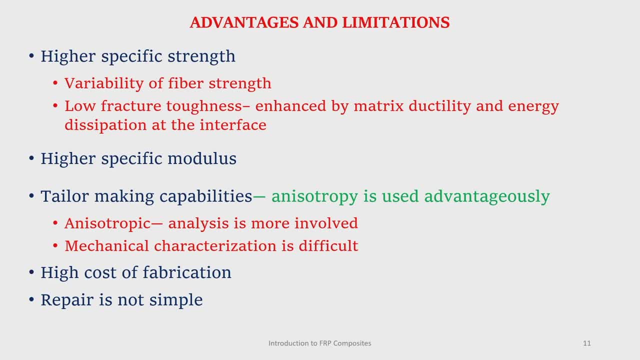 Then one important besides all this there is an important, I mean- advantage is tailor making capabilities. that means, we can actually tailor make the properties as per our requirement. how say for example: what do you mean by tailor make? here the anisotropy is used advantageously. 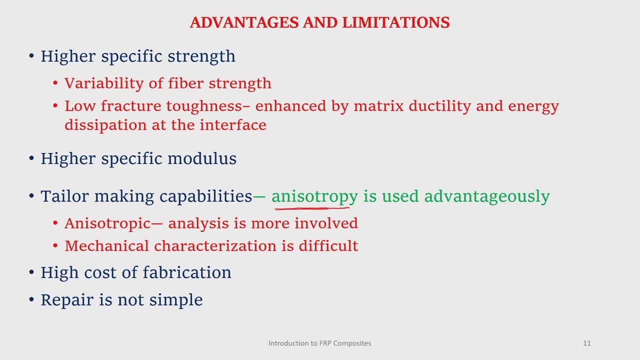 the term anisotropy we will discuss in details later on. the fibers are actually anisotropic. that means the properties are actually direction dependent. that means if you take a typical fiber you know it is longitudinal. that means along its axis, the strength And stiffness. suppose this is direction 1, so along its axis, the strength and stiffness. 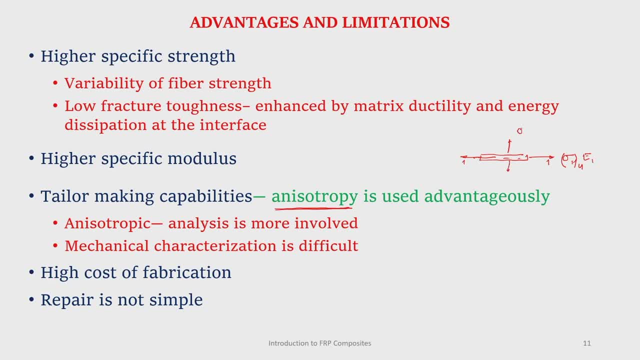 is far higher compared to that in the transverse direction. u 1 is much greater than e 2. strength in direction 1 is also greater than strength in direction 2, so this is anisotropy and this is used advantageously. Suppose we want a component which is supposed to take axial load. therefore we will choose. 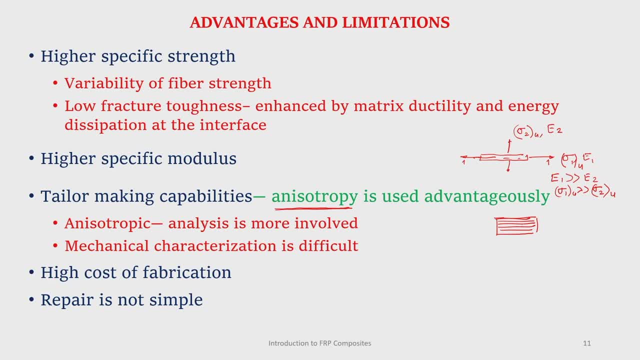 a fiber reinforced polymer composites where the fibers are in the direction of the load and it can serve but we do not require, suppose, the stiffness or strength in the other direction so high. suppose we want our desired u 1 by e 2 is, say is equal to 10.. 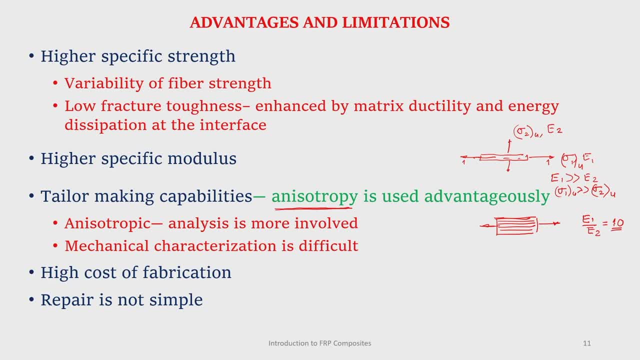 So we can actually tailor make that by choosing the reinforcement and the matrix and the relative proportion. that is very, very important. So another important aspect is in the example of tailor making is say, sometimes in space applications there are components may actually experience a temperature range, suppose anything. 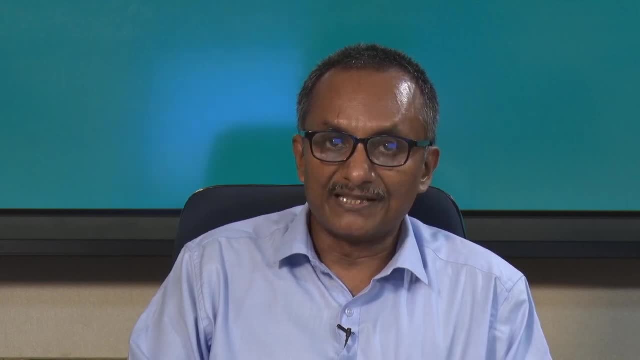 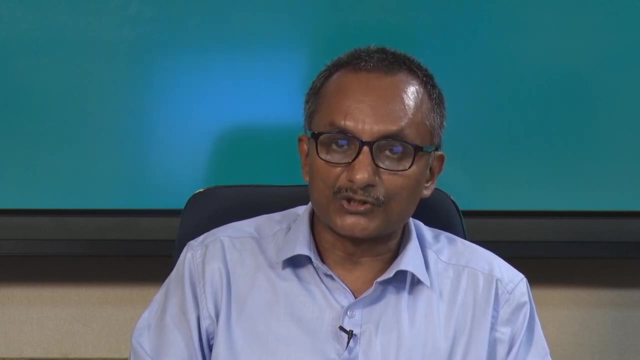 between minus 92 plus 100, 150 in that gamma at of temperature. you know, if you just go by the coefficient of thermal expansion, The shape distortion will be there, because if the temperature variation is so high, depending on the coefficient of thermal expansion, alpha there will be, you know, the dimension stability. 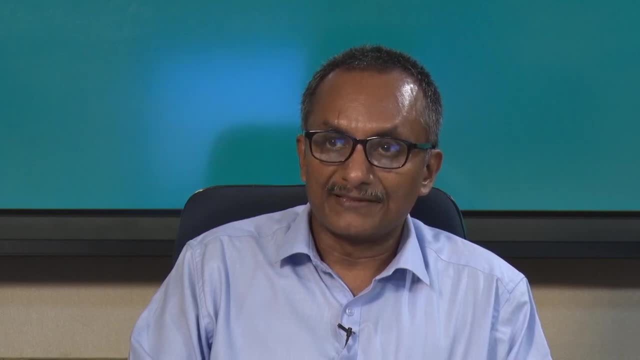 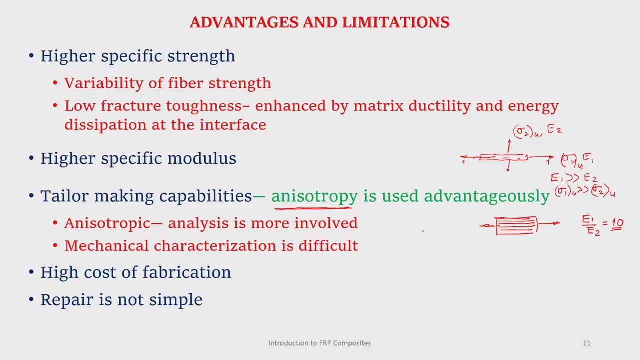 will not be there. but with composites it is possible that to choose the reinforcement and the matrix in such a way that some of may be the coefficient of thermal expansion in a particular direction- suppose coefficient of thermal expansion along in a particular direction- may be made almost 0 and thereby actually reducing the dimensional instability. 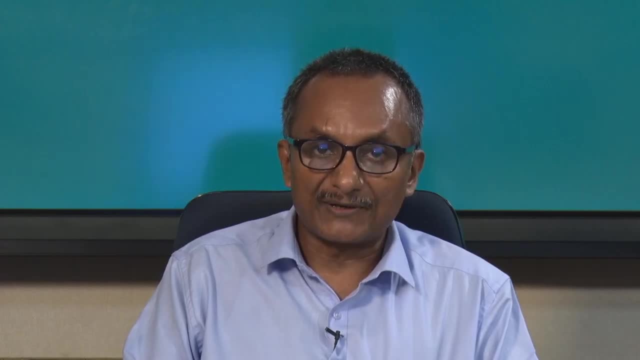 These are advantages, but anisotropy also has limitations. because it is anisotropic, the analysis is more involved compared to the isotropic materials. like, analysis of a component made of steel is much simpler compared to analysis of a composite which is made of anisotropic. 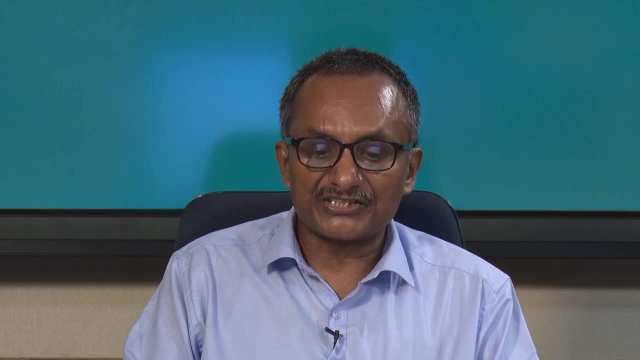 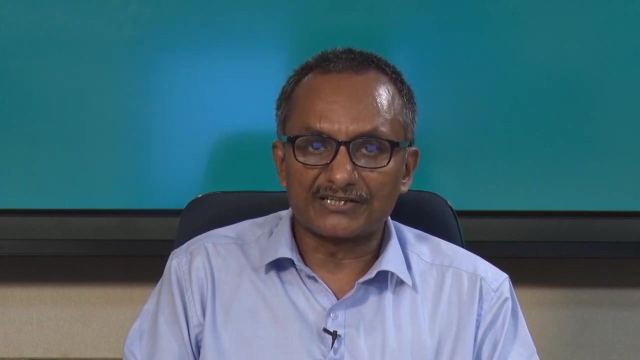 fibers and isotropic matrix. Okay, So mechanical characterization is difficult. okay, what do you mean by mechanical characterization? suppose, for example, if you actually want to characterize a material, suppose a steel, what we do? we make a sample, take it to the universal testing machine, load it, we can from. 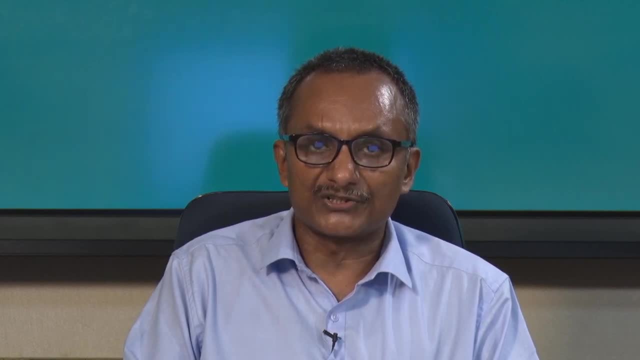 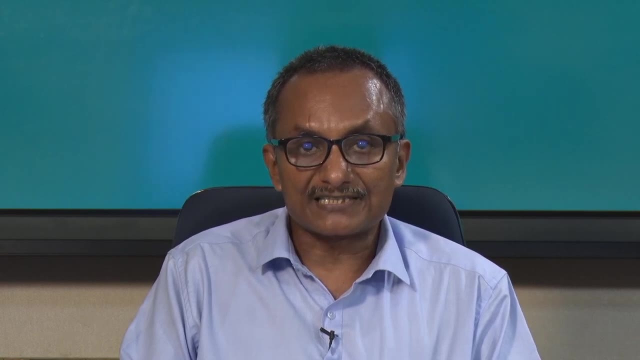 one single test we can find out what is its Young's modulus, what is Poisson's ratio and what is its, you know? and of course the residue modulus is a function of Young's modulus and Poisson's ratio. but it is not that straight forward in the case of composites. 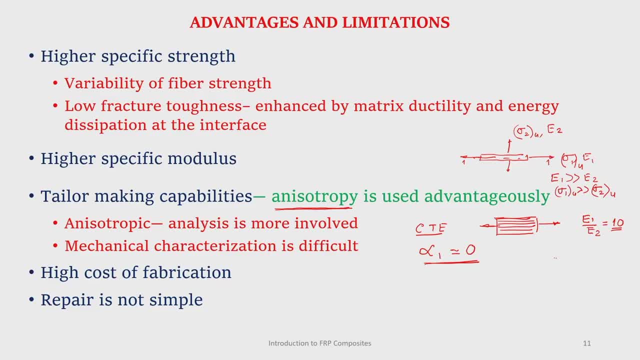 because it is an isotropic. that means in case of a component made of composites, I mean we have to find out Young's modulus along this direction. Young's modulus in this direction may be Young's modulus in the other direction similarly. So the mechanical characterization is not that straight forward and it is also difficult. 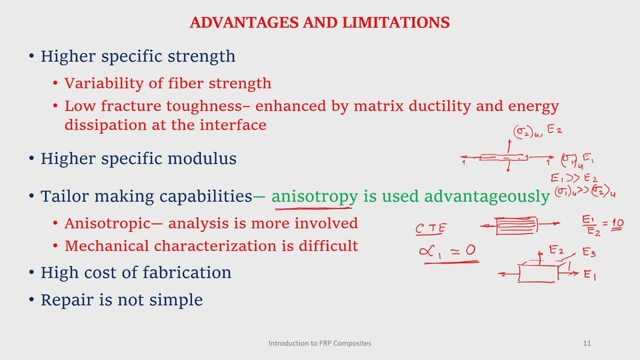 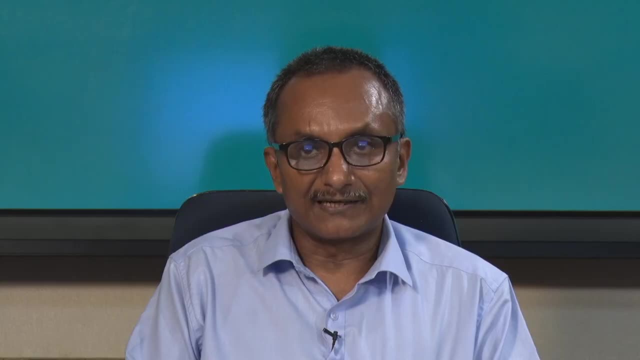 we will have a detailed discussion on this. when you do the mechanics Okay, And then coupling also, which makes it for the difficult, the mechanical characterization, then there is high cost of fabrications- okay. the manufacturing method is entirely defined, compared to that of, you know, conventional metallic materials and the cost of manufacturing. 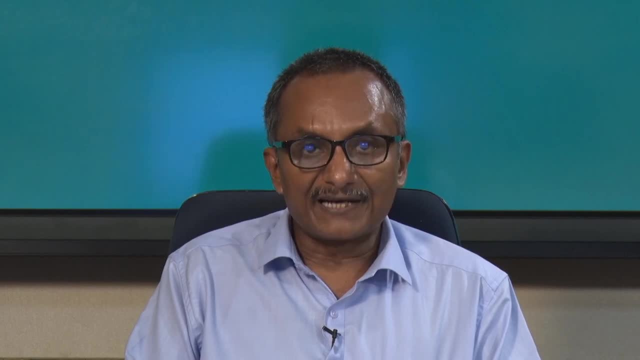 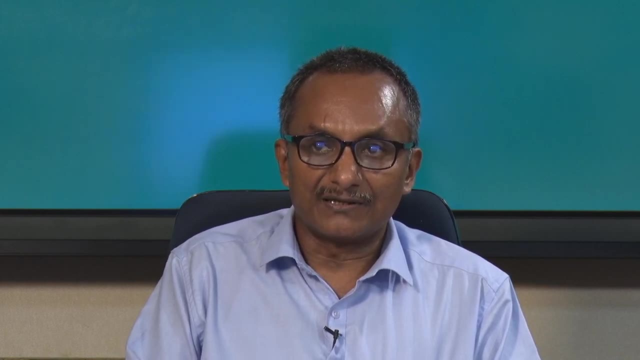 is still higher, but with mass production it is coming down and repair is not that simple like in case of conventional metallic materials. we can do welding, okay, we can do. it may not be if there is a flaw. it may not be that straight forward to repair a component. 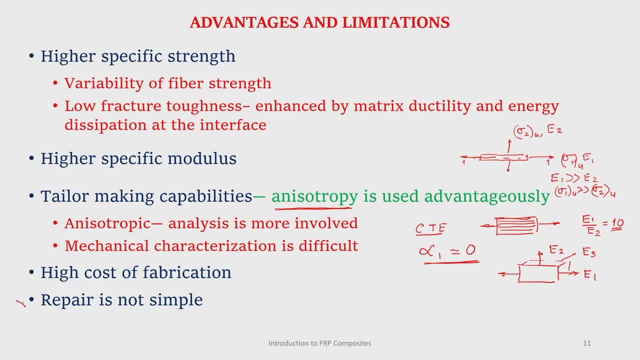 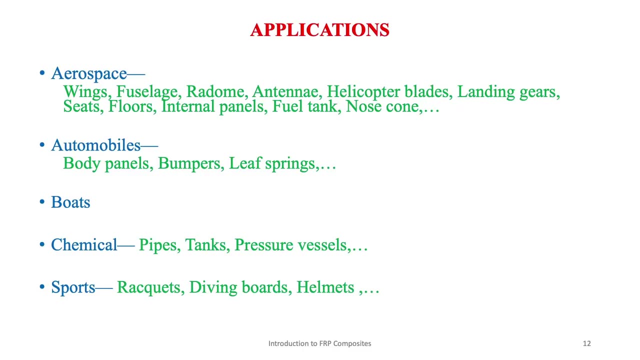 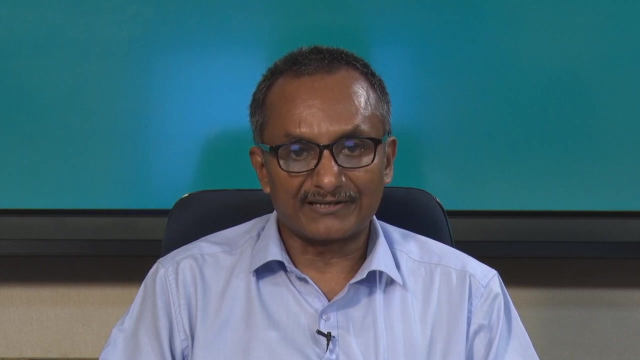 So these are some of the limitations. you know, these are some of the limitations. these are the advantages. Okay, Applications. I mean why we are actually studying this course. there are huge applications of composite material, especially the fiber reinforced polymer composite materials. If you look at aerospace structures, you know the wings, fuse lug, radome, antenna, helical. 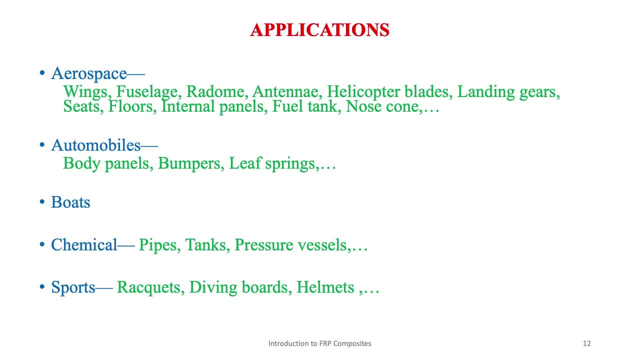 structure, Okay, Okay And so on. so many things are actually made of, you know, composite materials and therefore there are huge weight savings in this. aerospace structures, Then automobiles, body panels, bumpers, leaf springs- there are many such components. Boats are also made of fiber, glass fibers, you know.